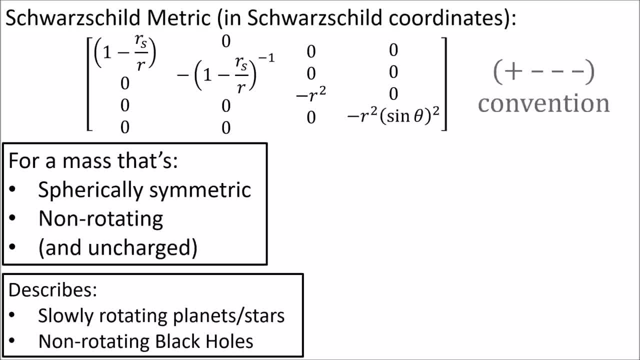 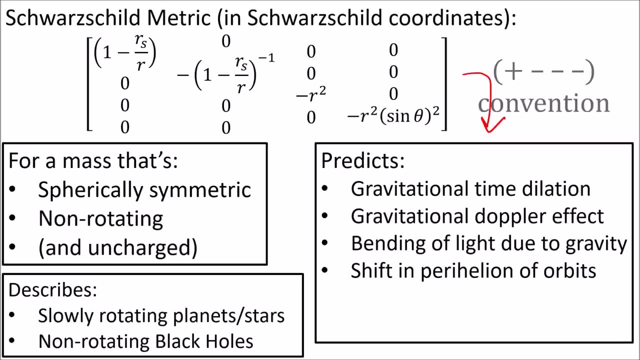 like planets and many stars. It's also useful for describing spacetime curvature near non-rotating black holes. The Schwarzschild metric predicts gravitational time dilation, the gravitational Doppler effect, the bending of light due to gravity shifting in the perihelion of orbits and the existence of black holes. 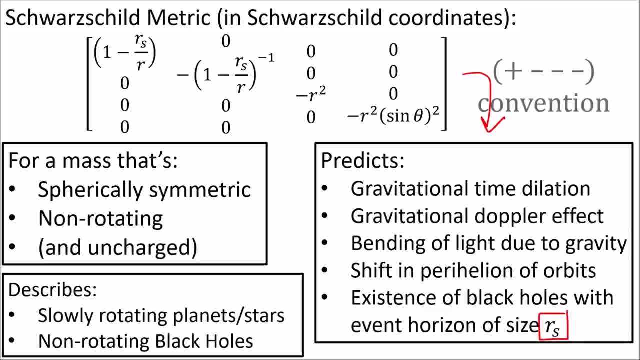 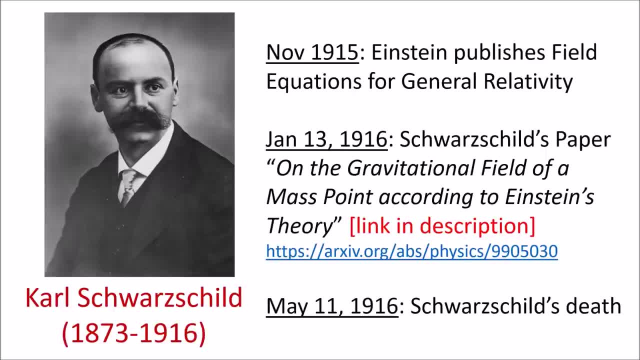 with uneventful gravitation. This metric is also called the Schwarzschild metric. The metric was first discovered by Karl Schwarzschild, who published it only a few months after Einstein's General Relativity paper in 1915.. Schwarzschild, unfortunately. 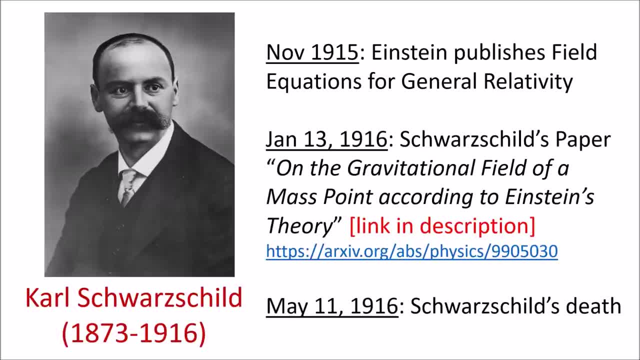 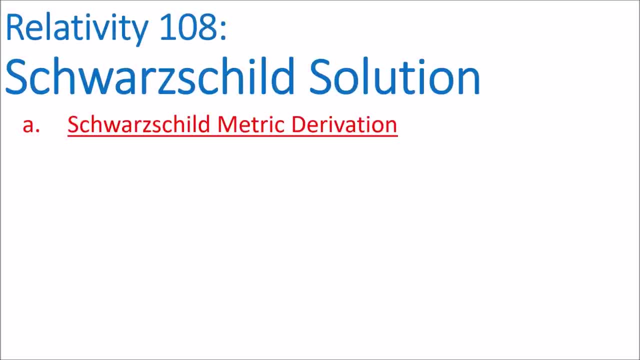 died only a few months later while serving in the German Army in World War I. In this video 108 we'll start by deriving the Schwarzschild metric from some starting assumptions. Then in 108 we'll interpret what the metric means explaining gravitational time dilation. 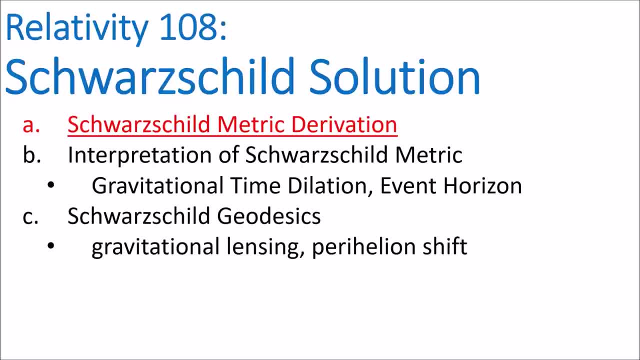 and also explaining a black hole's event horizon. In 108 we'll calculate the geodesics of the Schwarzschild metric which give the paths of light beams and massive bodies in the presence of gravity, which includes the perihelion shift of orbits. In 108 we'll cover some 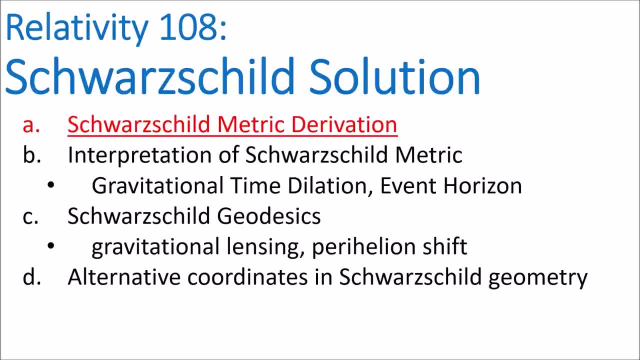 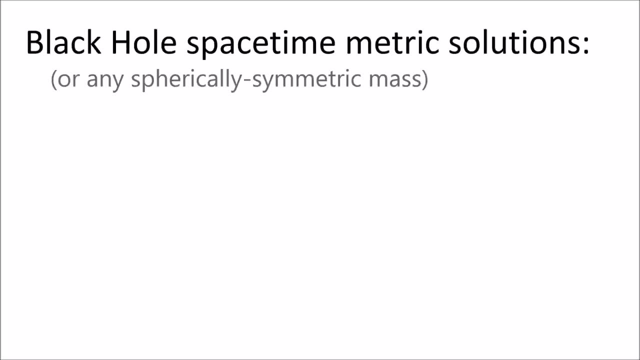 alternative coordinate systems for the Schwarzschild geometry that make it easier to understand, And in 108 I'll cover the gravitational doppler effect. I may also cover other topics like rotating black holes and the Kir metric later. When it comes to black hole solutions, we can categorize them for electrically. 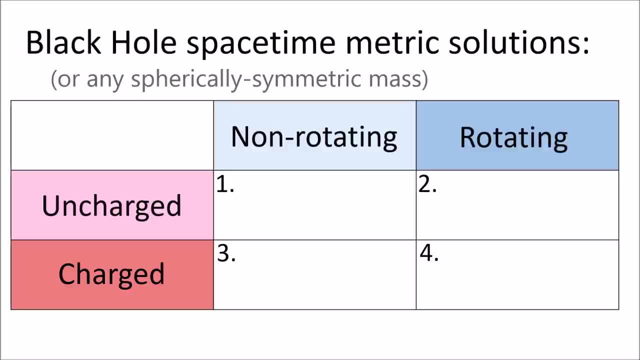 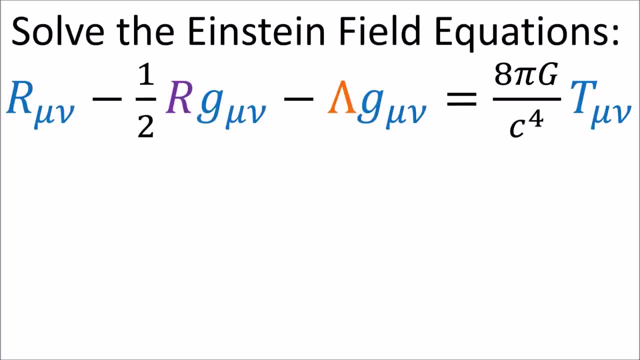 charged and uncharged black holes and rotating and non-rotating black holes. We're going to look at the uncharged, non-rotating case called the Schwarzschild solution equation. So we're now going to find the Schwarzschild solution to the Einstein field equations. 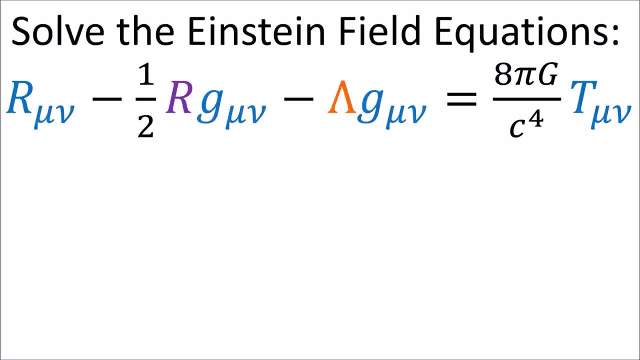 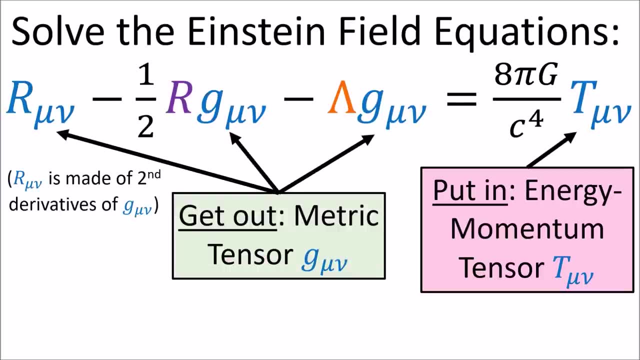 But what exactly does it mean to solve the Einstein field equations? It basically means we put in an energy-momentum tensor T and solve for the metric G. So we put in a description of the mass energy and momentum in spacetime and we get out. 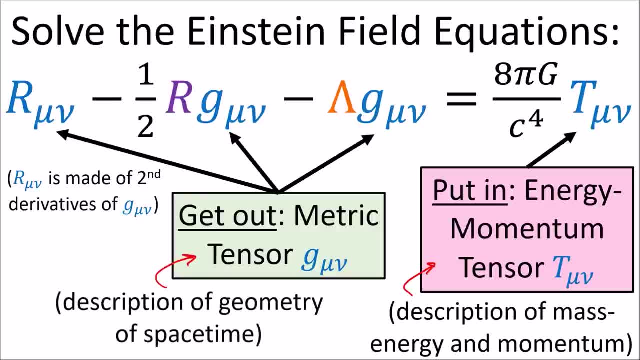 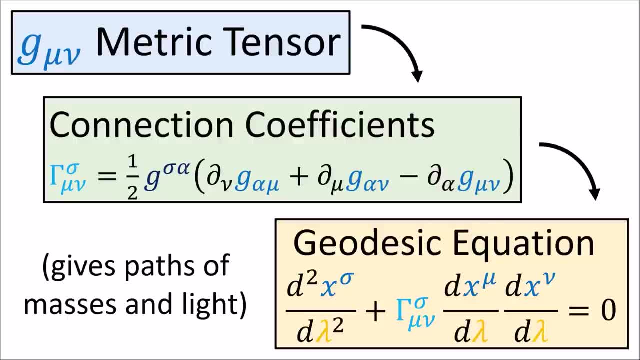 a complete description of the geometry of spacetime. Using the metric, we can then solve the geodesic equation which will give us the paths of massive objects and light beams through curved spacetime. So we'll know how gravity affects mass and light. 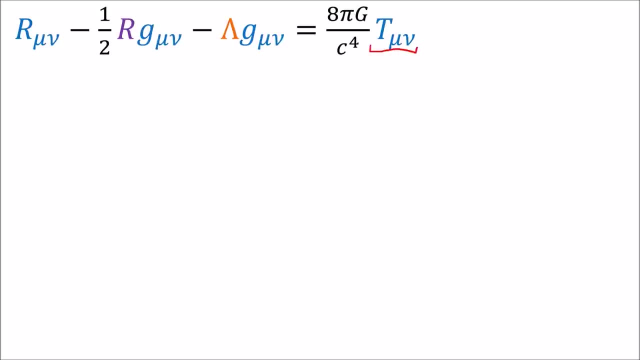 So what type of energy-momentum tensor will we use to get our spacetime solution for a spherically symmetric mass? Well, we know, inside the Earth we have mass and pressure, so the energy-momentum tensor inside the Earth is non-zero. 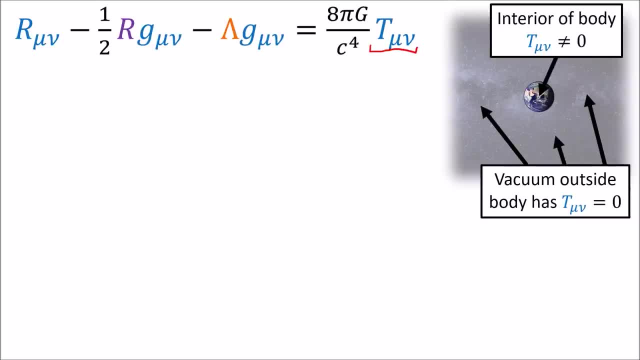 But outside the Earth we can assume spacetime is approximately a vacuum, So the energy-momentum tensor is zero. In this video we're just going to focus on spacetime in the exterior vacuum region only. So we're going to set the energy-momentum tensor in the Einstein field equations to 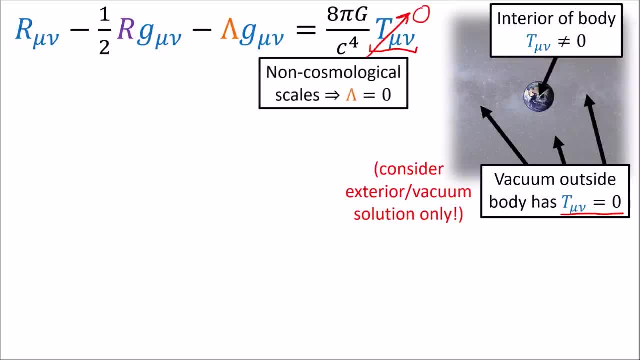 zero. We're also going to set the cosmological constant to zero, since it's basically negligible unless we're working at cosmological scales. Take the trace of what's left using the inverse metric to raise an index. The trace of the Ricci tensor is the Ricci scalar and the trace of the 4x4 identity. 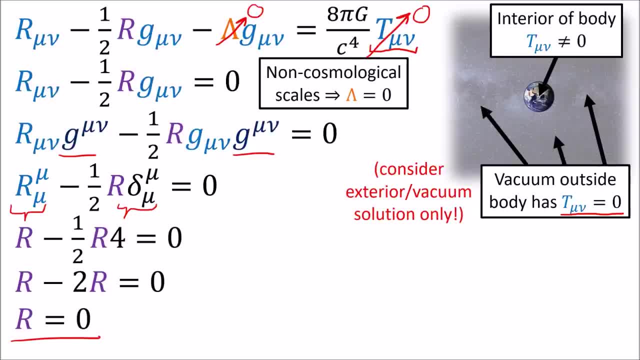 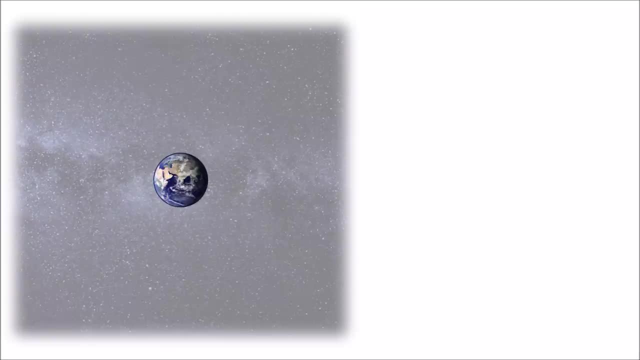 matrix is 4.. So we end up with the Ricci scalar being zero. So for a vacuum region, the Einstein field equations simplify to just the Ricci tensor being zero, which we call a Ricci flat spacetime. Now the vacuum outside the mass still involves curves. 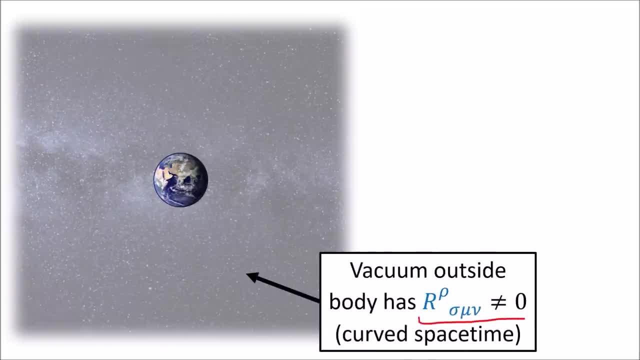 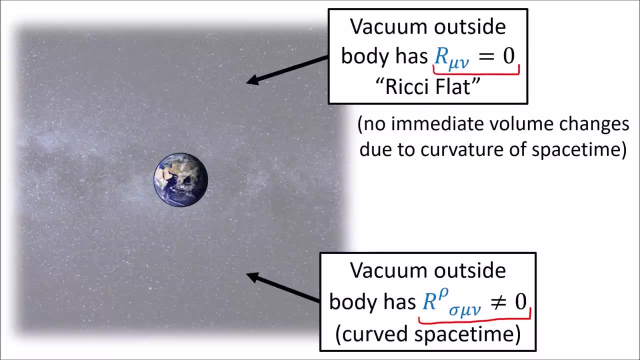 This is because the Riemann curvature tensor here is non-zero, But the Ricci tensor is zero And this means there are no immediate changes in the volume of a group of test particles outside the Earth as they move along geodesics. We only get tidal forces that squash and stretch the test particles without causing any immediate. 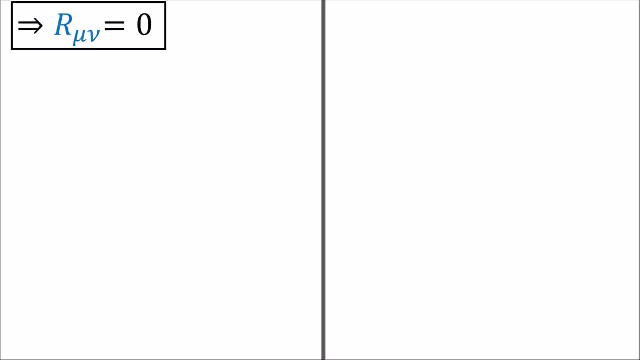 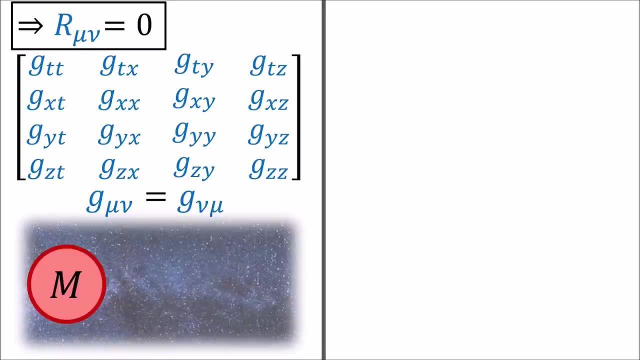 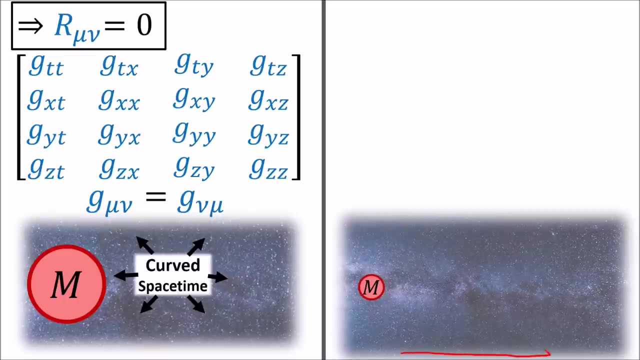 changes in the volume. So our job is to take this equation and solve for the components of the 4x4.. We're also going to assume that as we move far away from the mass, the effects of gravity become negligible and spacetime becomes basically flat, described by the Minkowski metric. 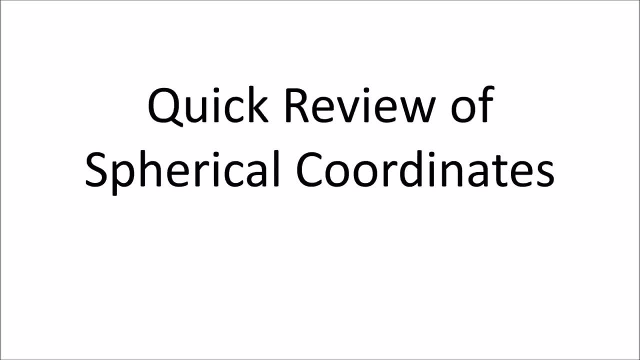 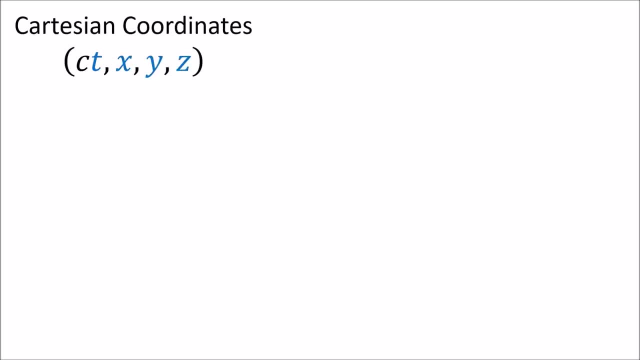 Now, before I start solving for the metric, I'm going to do a quick review of spherical coordinates. You can look at the video timestamps to skip this section, if you want. Since we're dealing with a spherically symmetric mass, it's better to deal with spacetime in. 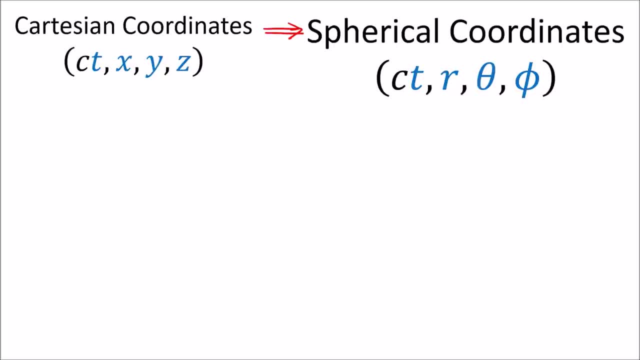 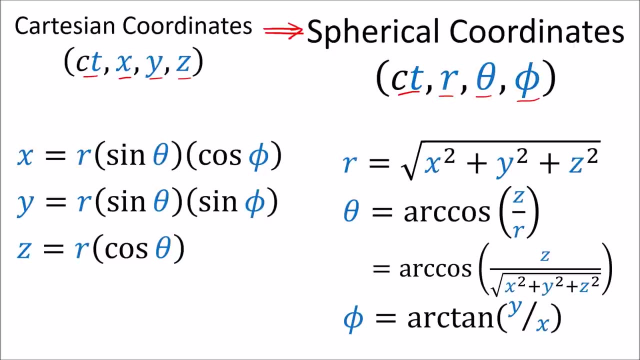 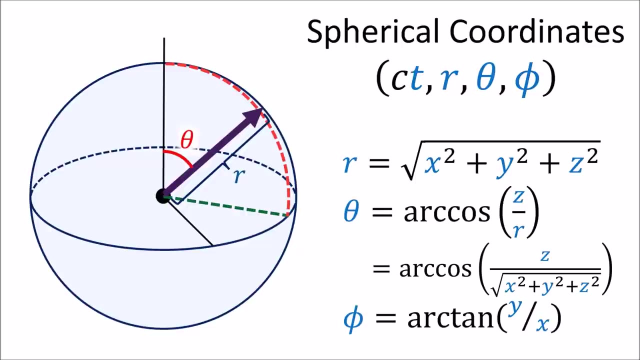 spherical coordinates. So instead of using the spacetime coordinates c, t, x, y, z, we'll use c, t, r, theta, phi, as defined here, Where r is the radius, theta is the angle from the north pole or co-latitude, and phi. 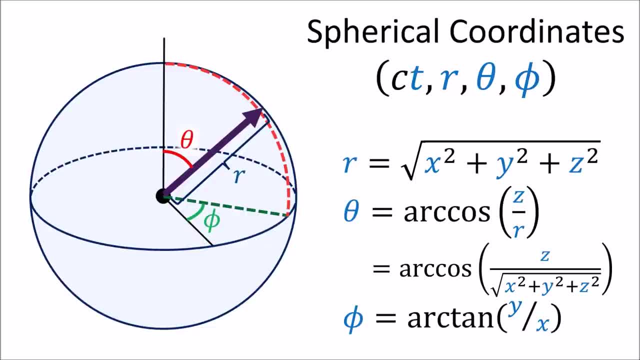 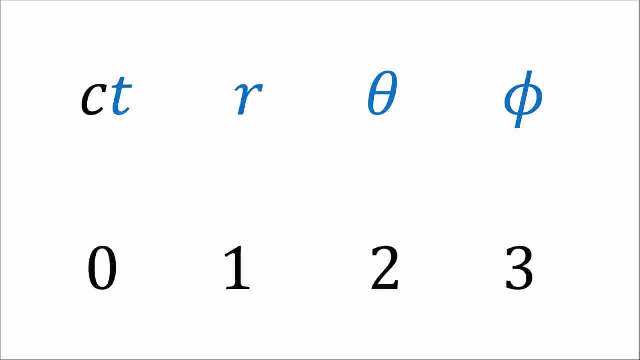 is the angle of rotation around the vertical axis or longitude. And, as a reminder, equations denote these four spacetime coordinates using the 0,, 1, 2, 3 indices, where 0 indicates time and 1,, 2, 3 are the spatial dimensions. 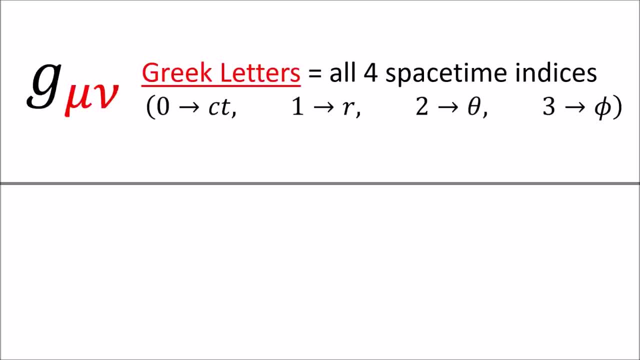 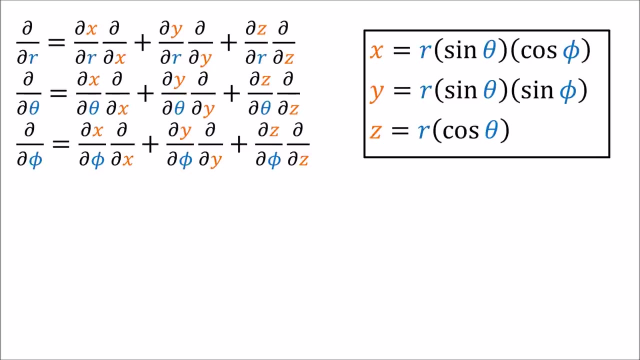 And in summations. when we use a Greek summation index, this refers to all four spacetime indices. But if we use a Latin or English letter for the summation index, this just refers to the spatial indices without time. If we change from the Cartesian coordinate basis to the spherical coordinate basis using 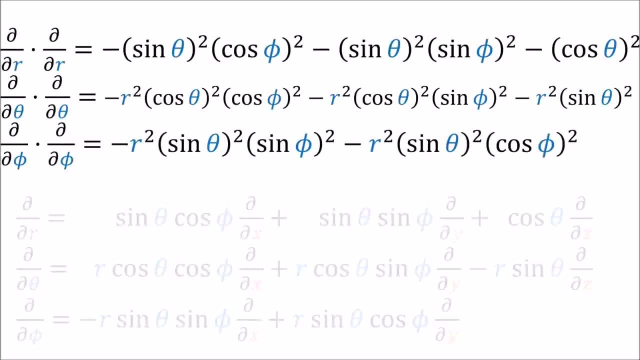 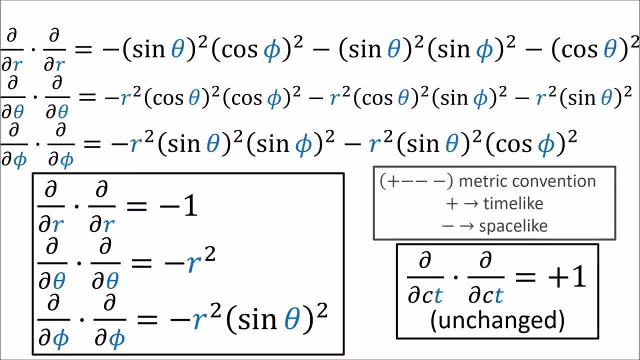 multivariable chain rule and calculate the dot products of the basis vectors. we get these components for the metric tensor in spherical coordinates. The spatial dot products have negative signs in front because in our mostly-minus convention for the metric space-like vectors have negative squared lengths. 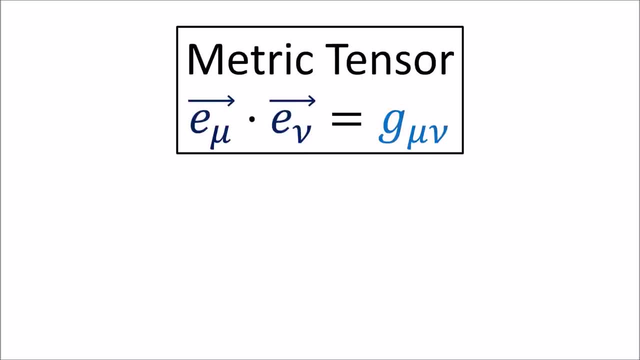 Remember, the components of the metric tensor are just the dot products of the basis vectors in our spacetime coordinate system. So the metric tensor helps us measure the space-time coordinates. So the metric tensor helps us measure the space-time coordinates. So the metric tensor helps us measure lengths and angles in spacetime. 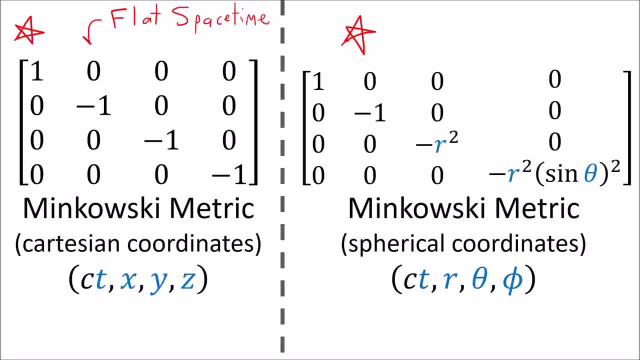 So both of these metric tensor matrices represent flat Minkowski space, But one is for Cartesian coordinates and the other is for spherical coordinates. The reason you see coordinate variables like r and theta in the metric components is because the theta and phi basis vectors change length depending on their position in space. 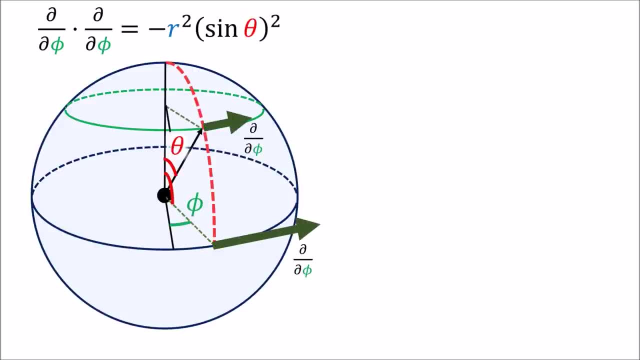 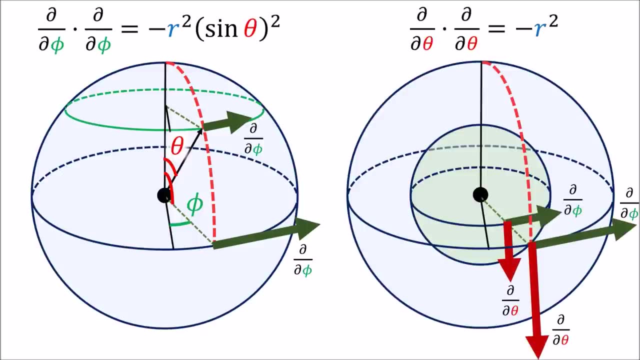 For example, the phi basis vector is bigger near the equator, And both the theta and phi basis vectors get longer as we move away from the origin. So this should be the metric far away from the mass as r approaches infinity and spacetime. 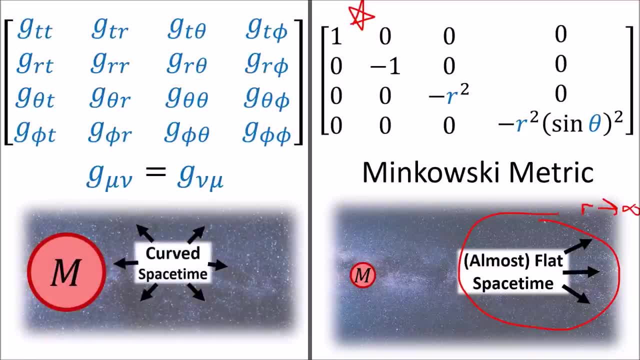 becomes flat But close to the mass. the metric components of the curved spacetime are unknown. We can use some assumptions to narrow down the exact form the metric components should take. First, we're going to assume that spacetime is static. The data is static. 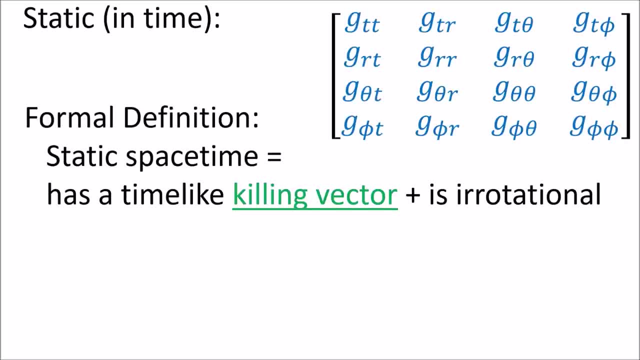 The data is static. The technically correct definition of static spacetime involves a concept called killing vectors, which I haven't covered yet, So I'm going to use a simplified definition. We'll take static spacetime to mean two things. First, the metric doesn't depend on time. 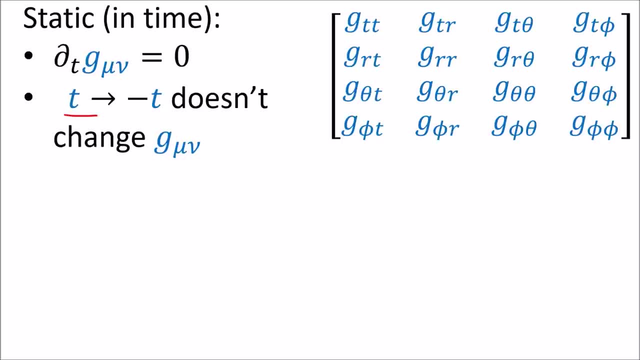 And second, that spacetime is symmetric. when we reverse the time coordinate. This is like mirror symmetry across the time axis. This guarantees the black hole isn't rotating. isn't rotating because if we reversed time for a rotating black hole, the gravitational 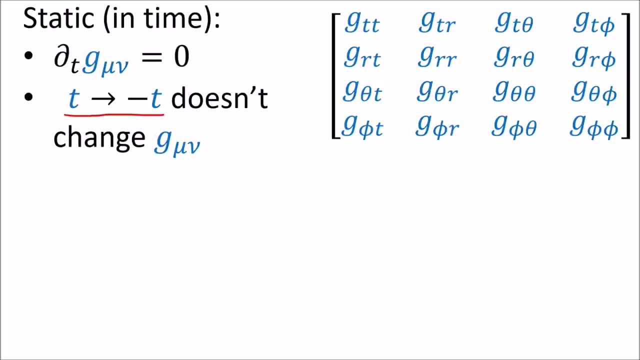 effects due to rotation would also reverse direction, Since basis vectors are just partial derivatives with respect to a coordinate variable. reversing the direction of the time coordinate also reverses the direction of the time basis vector. This does not change the GTT metric component, since the two new negative signs cancel out. 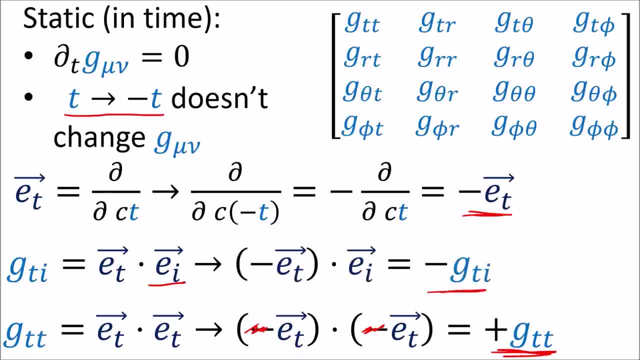 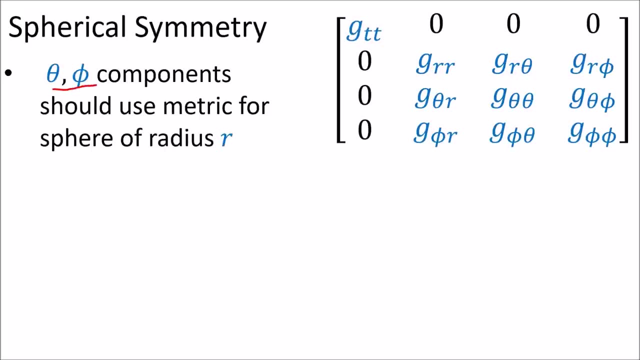 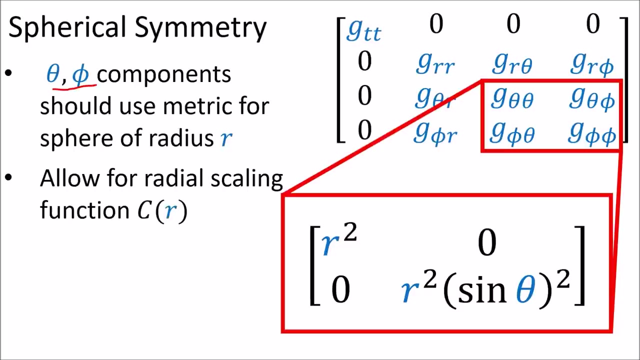 but it will change the sign of ET dotted with any of the EI space basis vectors. Since GTI equals negative GTI, these metric components go to zero. If we want spherical symmetry in space, the theta and phi components of the metric should resemble the metric for a sphere of radius R. However, we also allow multiplication by: 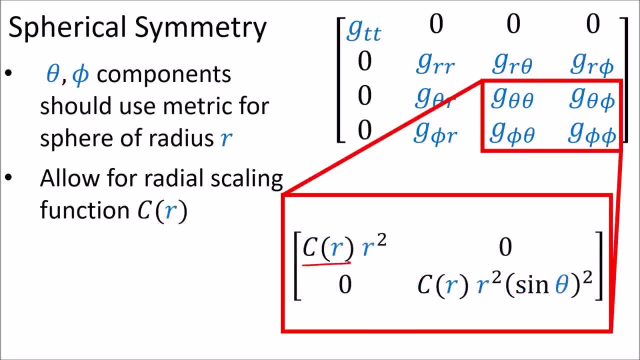 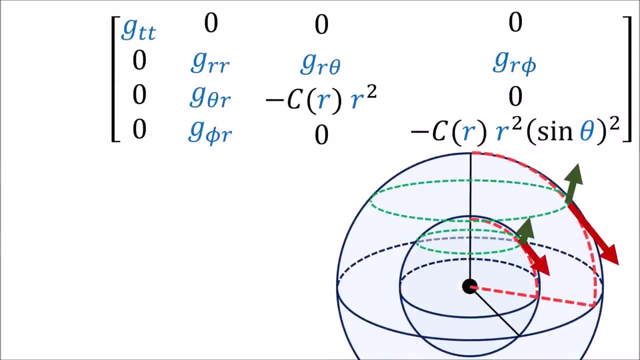 a radial function C, since this doesn't violate spherical symmetry. I'm also going to make these terms negative, since space-like vectors have negative metric components in the mostly-minus metric convention. If we want the radial basis vector ER to stick out normal to the sphere in the radial direction, 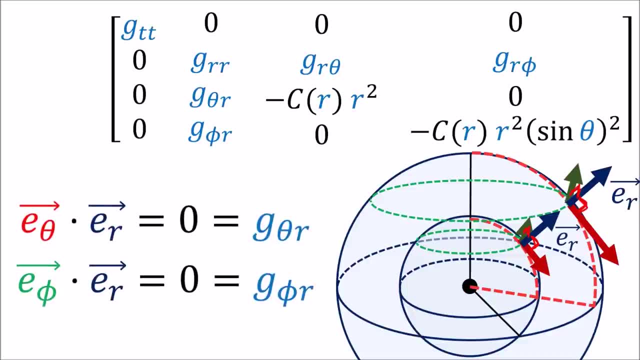 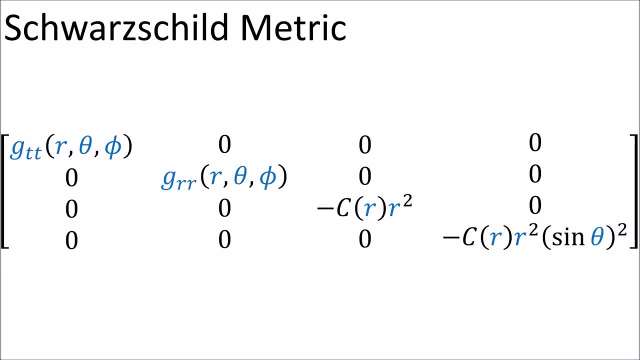 it must be perpendicular to both E-theta and E-phi. So these dot products and metric components go to zero. So under our assumptions so far, the metric is E-phi-phi-phi-phi-phi-phi-phi-phi-phi-phi-phi. 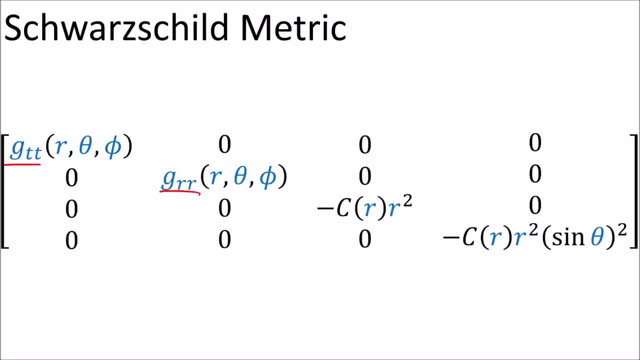 The remaining GTT and GRR components should only depend on the radial coordinate R if we want to maintain spherical symmetry. So we'll call them A-R and negative B-R. We're using a negative sign, since this metric component corresponds to a space-like direction. 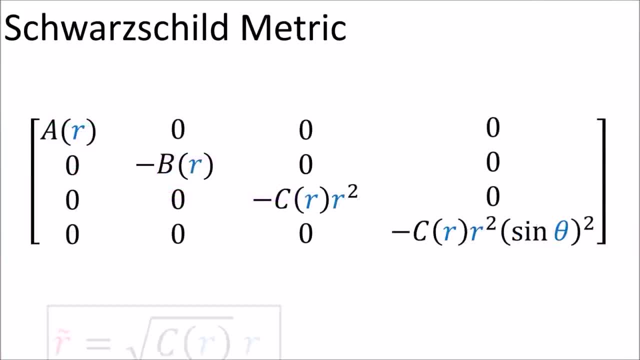 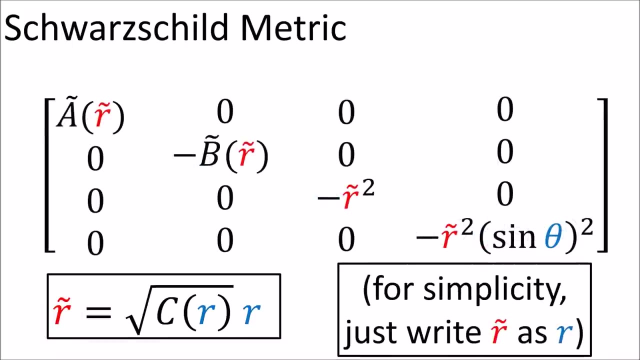 Now, to simplify things, we can always redefine the radial coordinate R to be: R-tilde equals R times the square root of R, And this would eliminate the function on the last two metric components. However, I'm not going to bother writing out R-tilde everywhere, so I'm just going to rewrite. 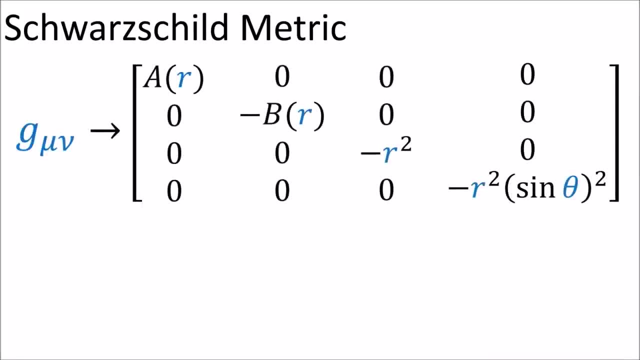 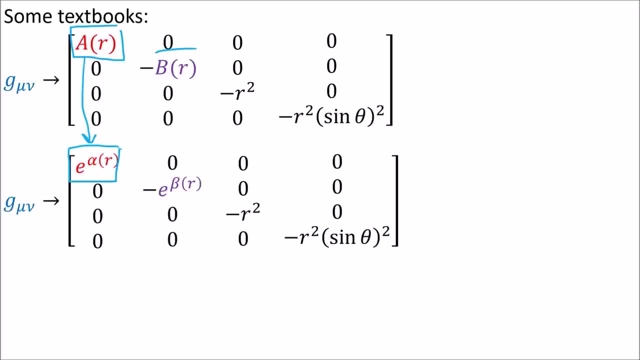 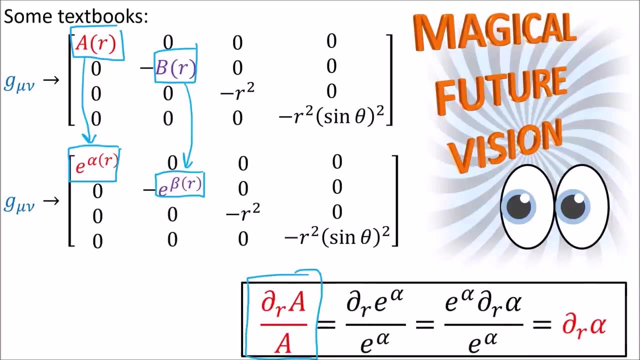 the new radial component as R instead. Just as a warning, some texts might write these A and B functions as exponential functions instead. They do this because they already know that getting the right answer involves using terms like partial A over A, Which becomes much simpler. 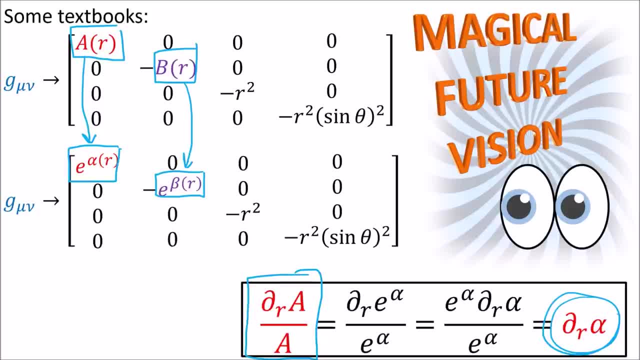 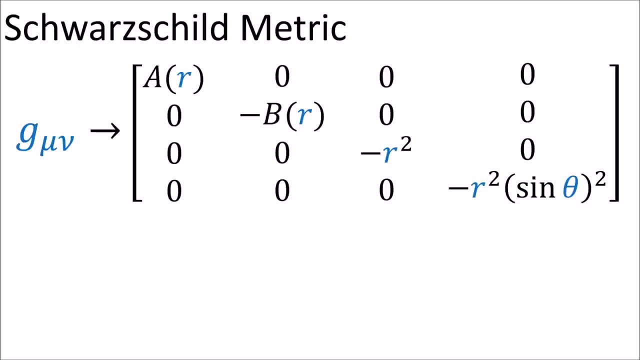 If you use exponential functions, But I'm not going to bother using this exponent trick in this video. So we've simplified the form of the metric as much as possible. In order to solve for A-R and B-R, we'll have to calculate the connection coefficients. 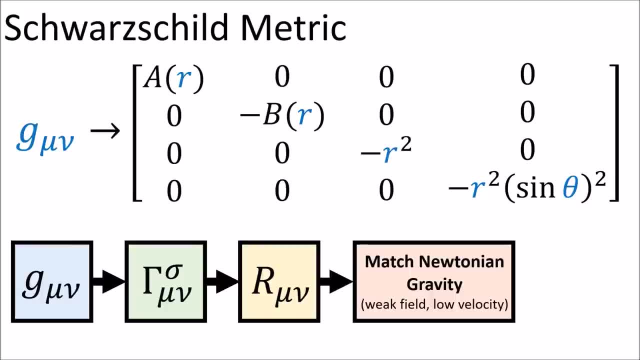 calculate the Ricci tensor components and then force the metric to give us the results of Newtonian gravity in the limit of low velocity and weak gravity, And this will give us the Schwarzschild metric. So let's start by calculating the connection coefficients. 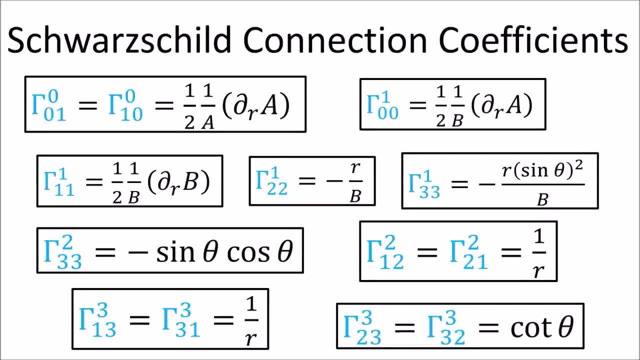 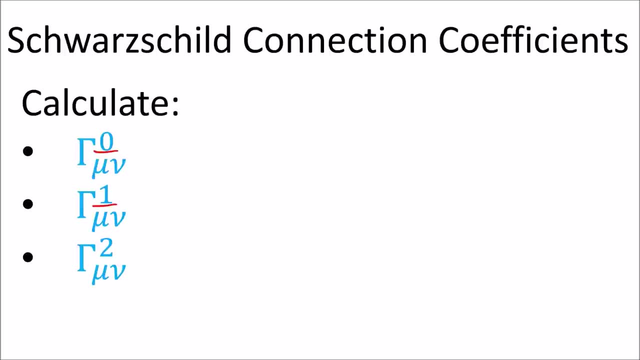 There are 13 non-zero connection coefficients in the Schwarzschild solution And only 9 of them are independent. Calculating them is pretty boring but necessary. I'll start by solving for the connection coefficients with a 0 upper index, then a 1 upper index. 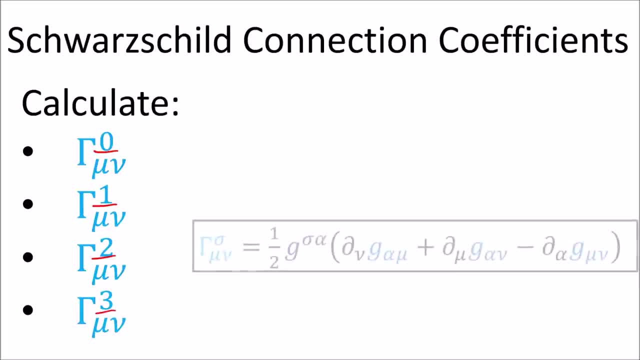 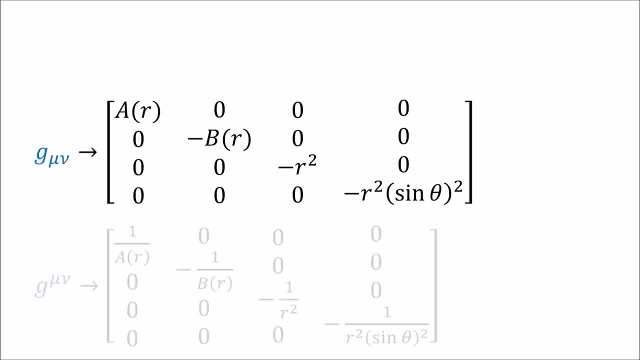 then the 2 and 3 upper indices. So here's the statement, Here's the result, Here's the standard formula for the connection coefficients. Since the metric is diagonal, we can easily get the inverse metric just by taking the reciprocal of all of the diagonal elements denoted by G with the upper indices. 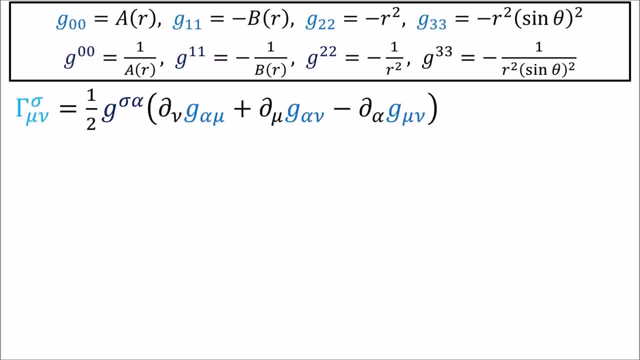 So here's the standard formula for the connection coefficients. But since we know that our metric is diagonal, its two indices always need to match if the components are to be non-zero. So we can rewrite the sigma-alpha inverse metric with repeated sigma-sigma indices to make. 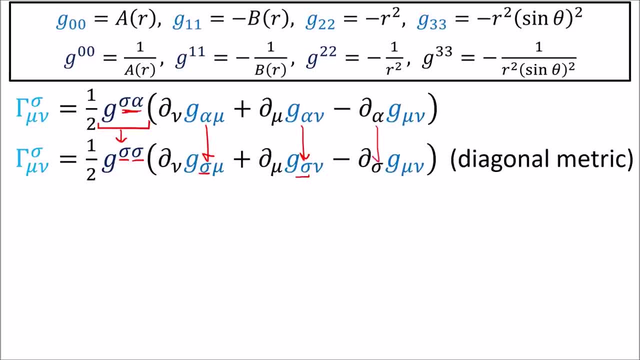 it diagonal and replace all other alpha indices with sigma. So this is not a summation over sigma here, It's just denoting that these two indices always need to be the same. Now let's look at the connection coefficients with 0 on top. 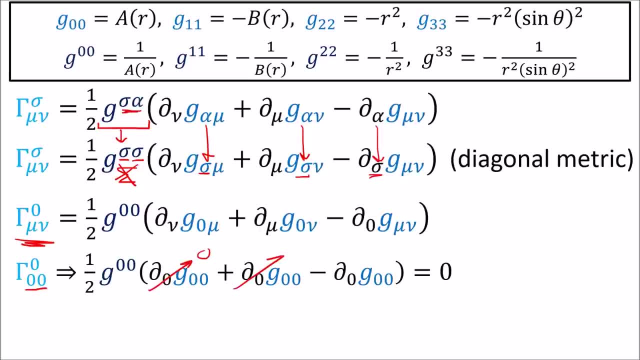 With 0, 0 on the bottom, all the time derivative terms go to 0. Since G doesn't depend on 0. So we can rewrite the sigma-alpha inverse metric with repeated sigma-sigma indices to make it diagonal on time, so we get zero. 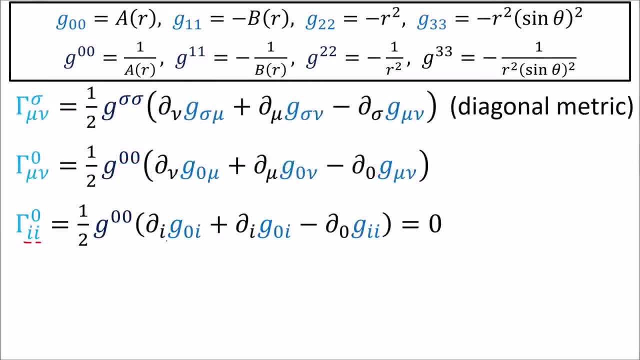 If both the lower indices are the same spatial index i. these metric components here are not diagonal elements of the matrix and therefore they must be zero From now on. I'm just going to cross out non-diagonal metric components without saying anything out loud, since it's going to happen a lot. 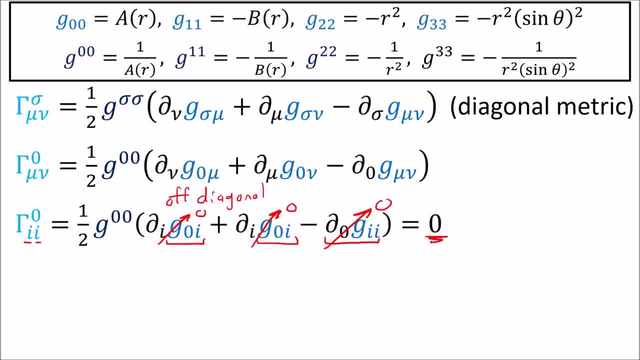 This time derivative term is zero, since the metric components don't depend on time And if the lower indices are both spatial but not equal, all the metric components are off-diagonal, so we get zero. In the case where one lower index is time and the other is spatial, this term survives. 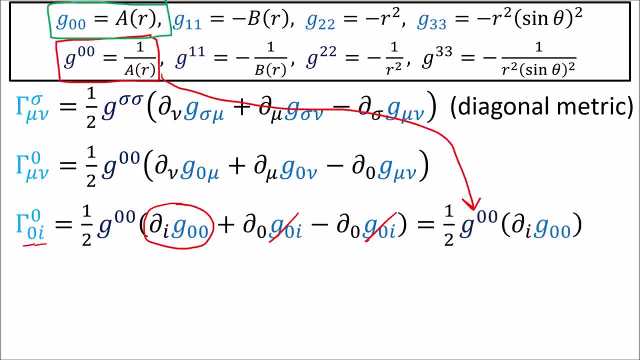 g inverse zero. zero is one over a and g zero zero is just a. This spatial i derivative can be any of partial one, partial two or partial three, or in other words partial r, partial theta. Since the a function only depends on r, only the partial r term gives a non-zero result. 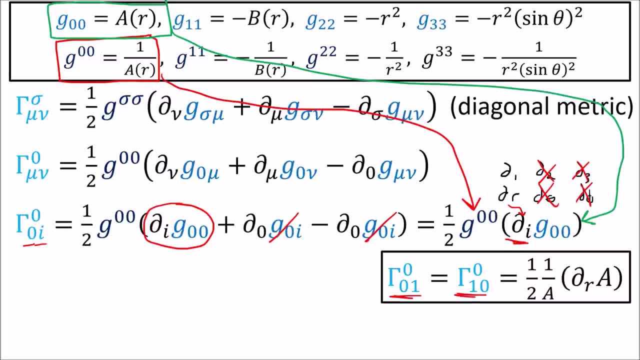 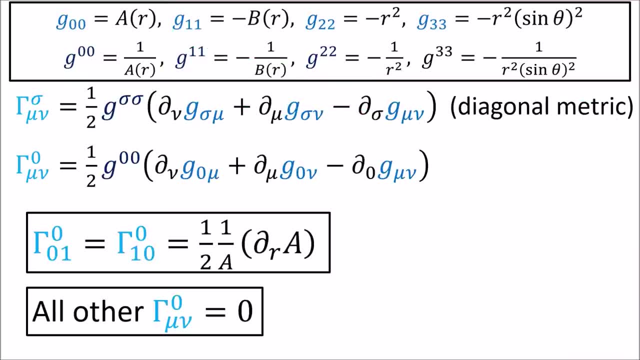 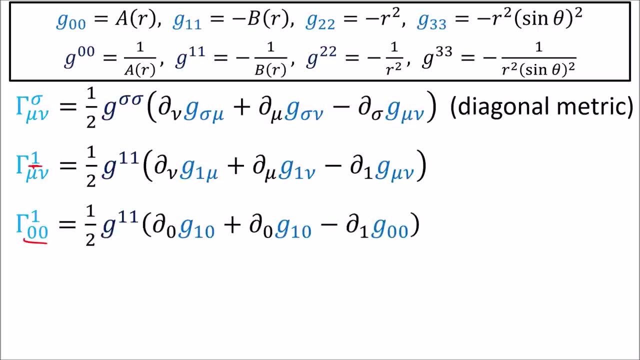 So the lower zero, one and one zero coefficients are non-zero, But zero two and zero three go to zero. So those are all the connection coefficients with a zero index up top. Now let's continue to the coefficients with a one on top For zero, zero on the bottom. 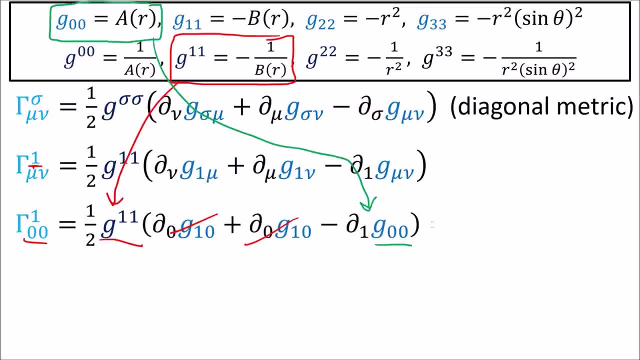 We get negative one over b here and the r derivative of a giving this For one one on the bottom. These cancel and we get negative one over b times the r derivative of negative b With two, two on the bottom. 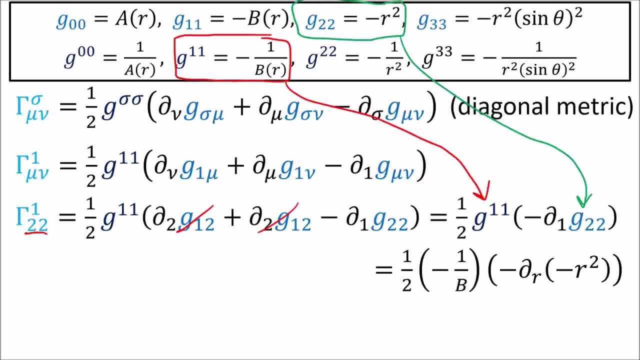 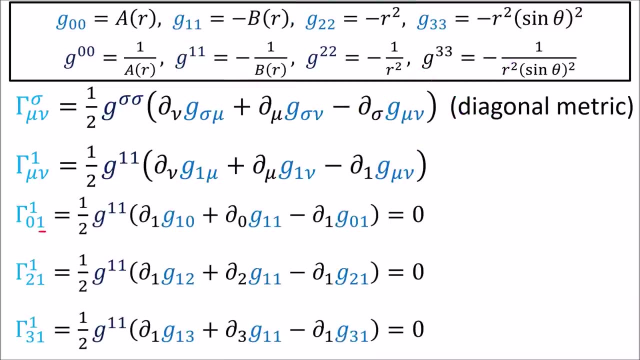 We get negative one over b and the r derivative of r squared, which is just two r. So we get negative r over b. And for the three, three on the bottom, We get the same thing multiplied by sine squared. When one of the lower indices is one, all the coefficients go to zero either, because 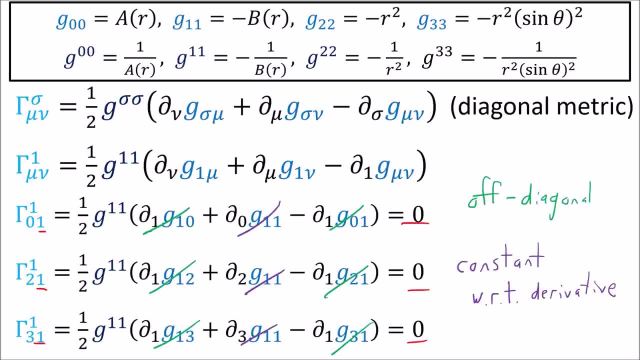 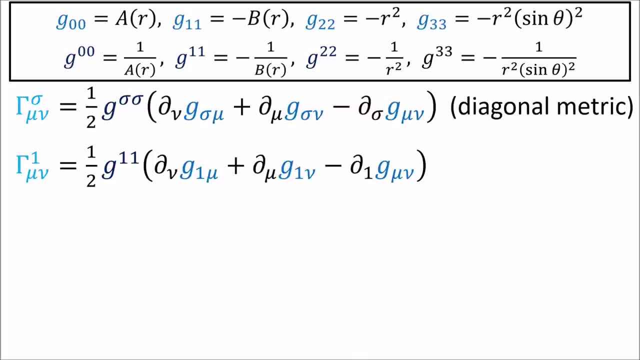 they are off diagonal or constant with respect to a derivative. Any other mixed lower indices give all off diagonal metric components, so they go to zero too. So these are all the non-zero coefficients, with one on top. For the two on top coefficients: 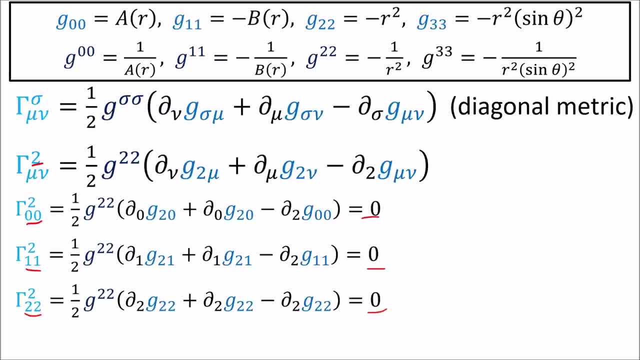 0, 0, 1, 1, or 2, 2 on the bottom all give 0. But 3, 3 on the bottom gives us negative 1 over r-squared for the inverse 2, 2 components. 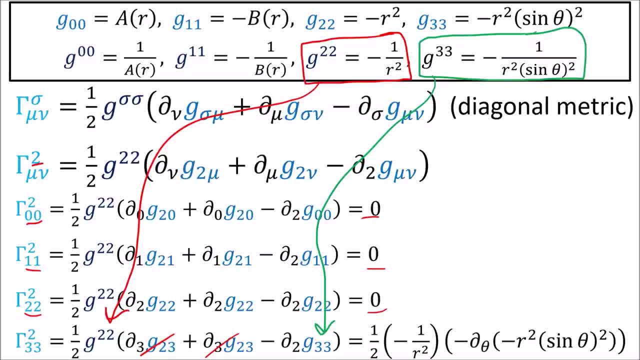 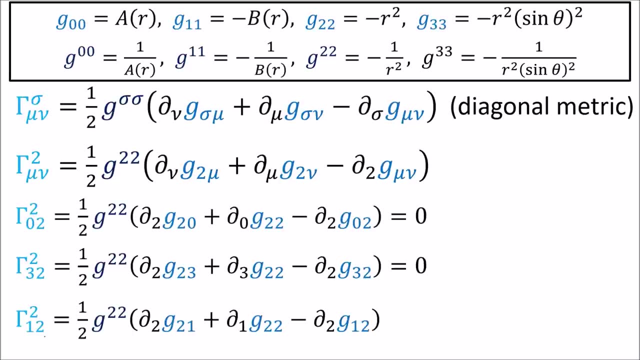 and the derivative with respect to theta of the 3, 3 component, The negative 1 over r-squared and negative r-squared cancel, and the derivative of sine-squared is 2 sine times cosine. If one of the lower indices is 2,, then having 1, 2 on the bottom gives us a non-zero term. 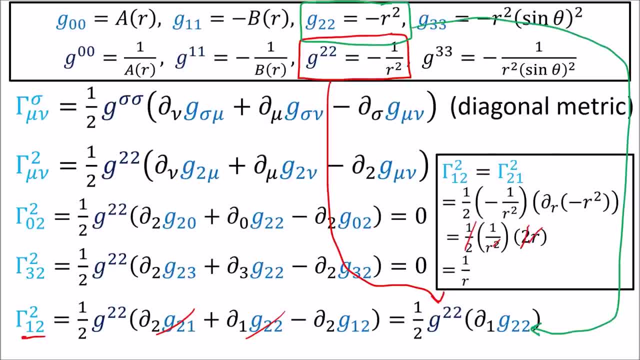 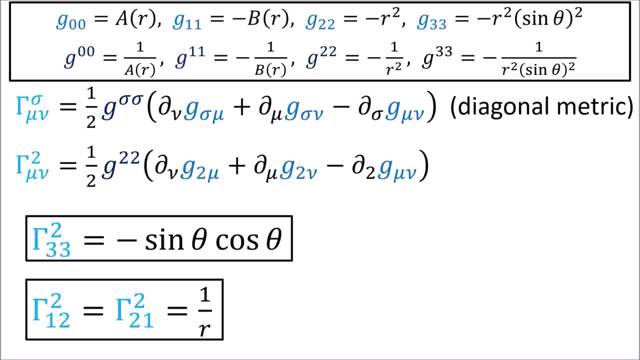 which simplifies to 1 over r. Any other mix of indices on the bottom all go to 0. So these are all the non-zero coefficients with 2 on top. Finally, for the 3 on top coefficients, if we have repeated lower indices that are not, 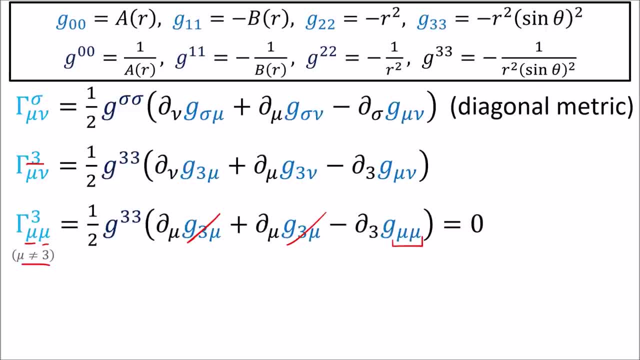 3, the off-diagonals go to 0.. And the last term goes to 0.. Since the metric is 0, the off-diagonals go to 0.. The metric components don't depend on phi, And the 3,- 3 lower indices go to 0 as well, because nothing depends on phi. 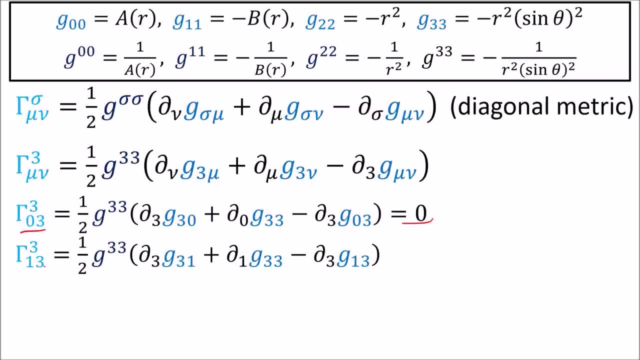 For 0, 3 on the bottom, we get 0.. For 1, 3 on the bottom, we get the derivative of g, 3, 3 with respect to r, which is non-zero. Cancelling sine-squared and churning through the derivative and algebra, we get 1 over. 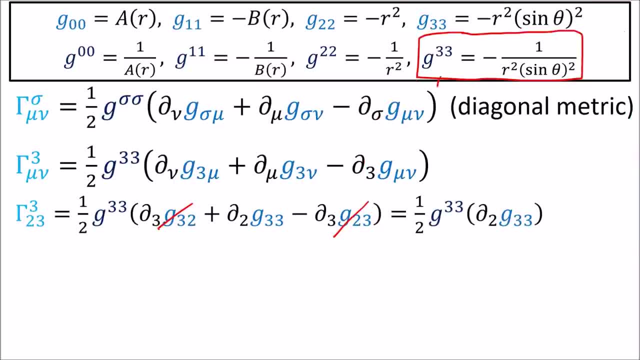 r For 2, 3 on the bottom, we get 1 over r For 3, 3 on the bottom. g 3, 3 depends on theta And cancelling r-squared and working through gives us cosine over sine, which is the definition. 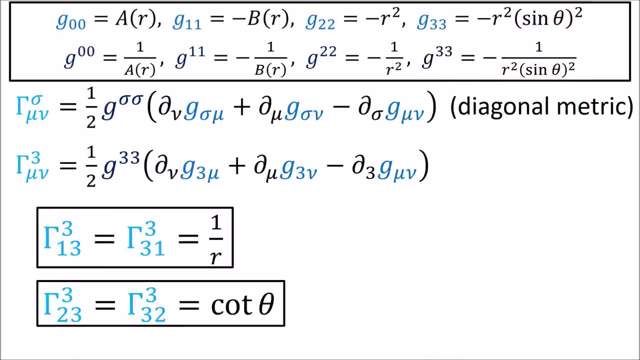 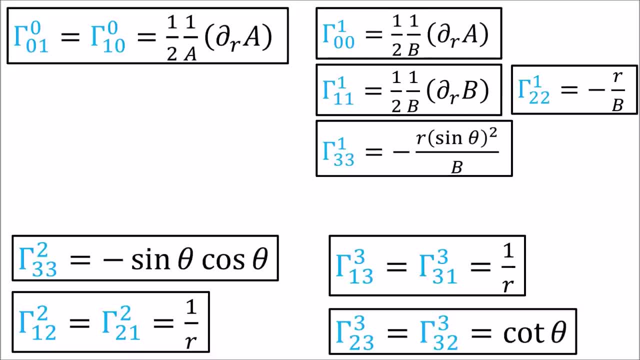 of cotangent. All the other mixed lower indices go to 0.. So now we have all 9 of the independent non-zero connection coefficients And even though I'm using the mostly-minuses metric, all of these coefficients should be the same in both the mostly-minus and mostly-plus coefficients. 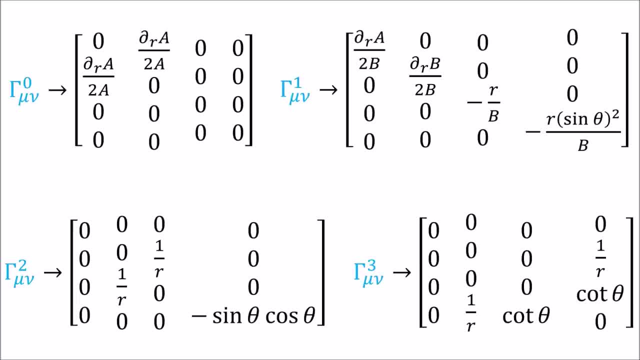 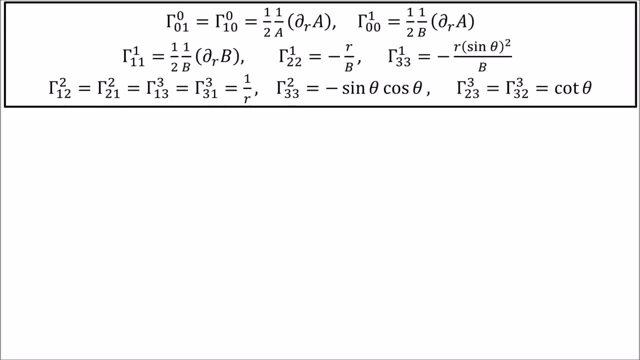 If you want to view these connection coefficients as arrays, they would look like this. So, given these connection coefficients, we're now going to calculate the formulas for r0,, 0,, r11, and r22.. Remember, our Einstein field equations tell us that all the components of the Ricci tensor 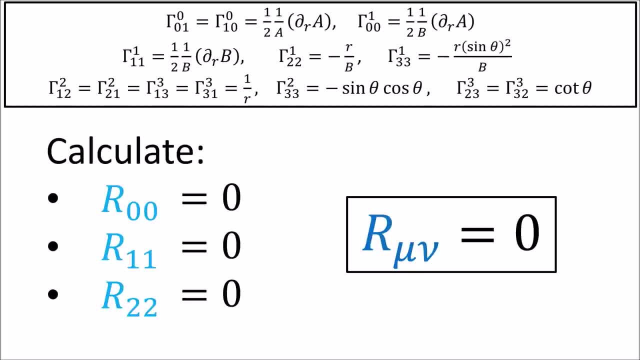 are equal to 0. But it is important to remember that all the components of the Ricci tensor are equal to 0. So we will likely have to work on these three equations in more detail. We will see that these three equations will be enough to solve for our a and b fields. 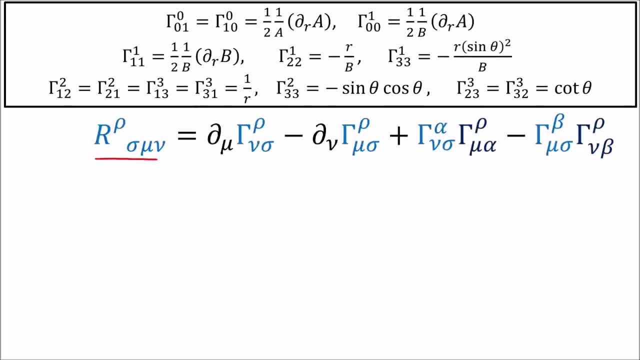 functions. Remember, given the Riemann tensor, the Ricci tensor is just the Riemann tensor with its upper and lower middle indices summed together, So the 0,0 Ricci component looks like this. Now there are a lot of summations here, like the summations over mu, alpha and beta, but it will. 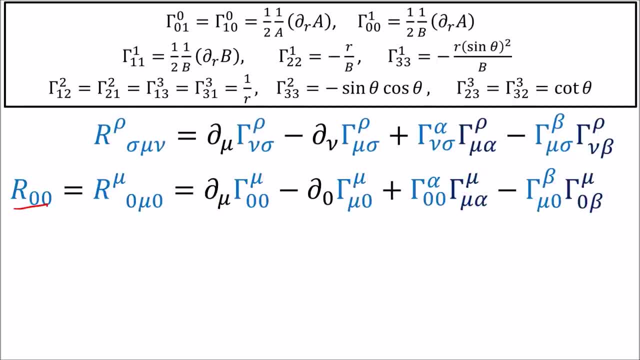 turn out. a lot of these summation terms go to zero For each of the four terms. here we need to look at the non-zero connection coefficients and decide what the non-zero coefficients in these summations are. For example, the first term has two zero indices on the bottom of the connection. 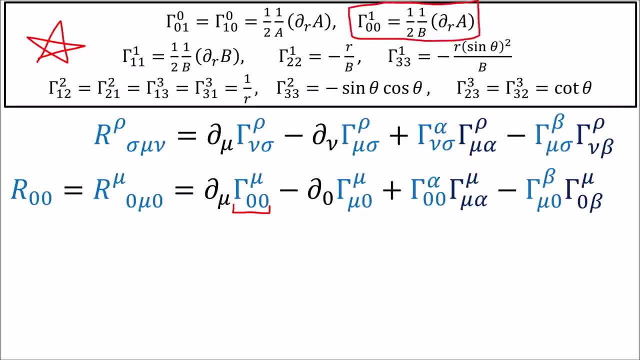 coefficient and there's only a single non-zero connection coefficient with two zero indices on the bottom, which is the 1,0,0 coefficient. So this means that even though the mu index is technically summed from 0 to 3,, only the mu-index is technically summed from 0 to 3.. 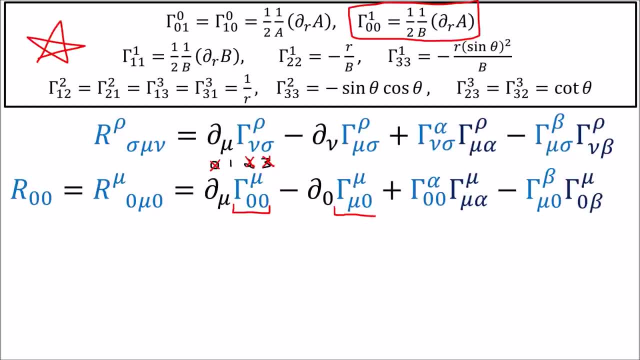 The second term has no coefficients, with zero on the lower right, with the other two indices matching, so it goes to zero. For the third term, looking at the alpha index, with two zeroes on the bottom, alpha must be 1 for this to be non-zero. And for the fourth term, looking at the beta index, 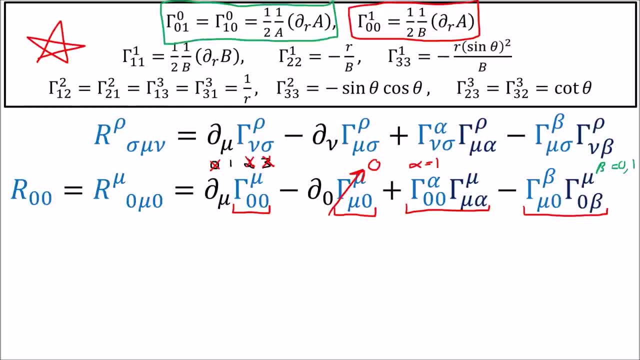 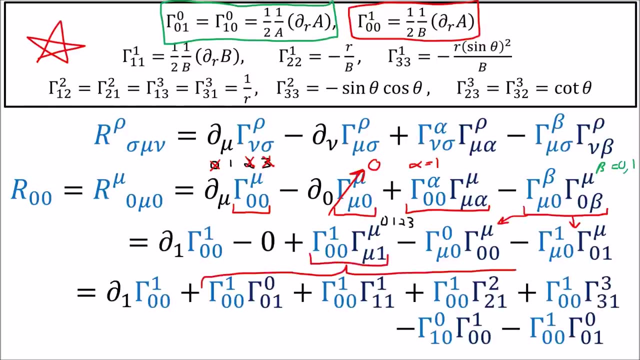 we see that beta could be 0 or 1,0,0. But not 2 or 3.. So the beta summation expands to two terms. We still have some mu summations left Here. mu could be either 0,, 1,, 2, or 3.. So this expands to four terms. 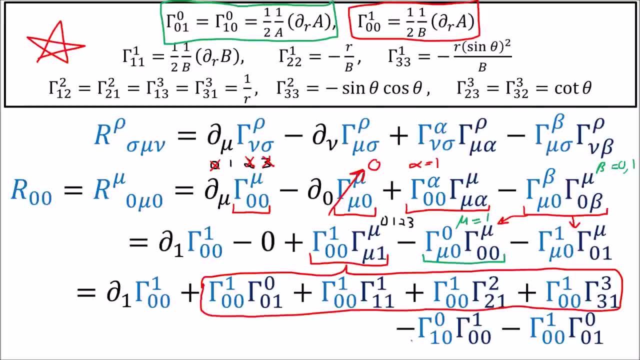 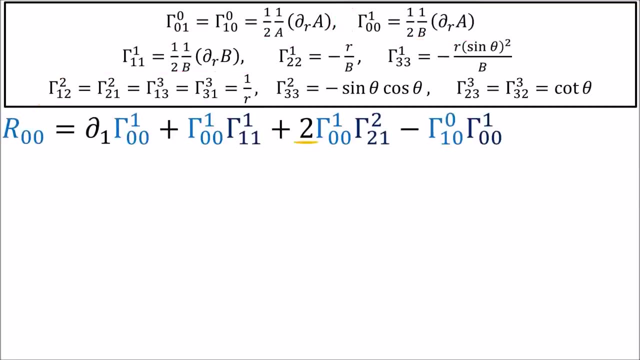 For the last two summations, mu must equal 1 in the first summation and mu must equal 0 in the second summation. Now this conveniently cancels with this, and since the mu-1 and 3, 3, 1 coefficients are equal, I'm going to group them as two times the same term. 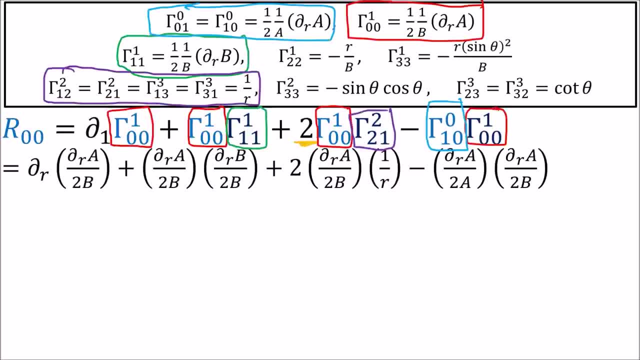 We're now ready to sub in the formulas for the connection coefficients. Most of these we can just multiply together. But this derivative term with the 1 coordinate, which is the r coordinate, involves product rule for the product of partial rA and the reciprocal of b. We get the second partial derivative of a in the first term. 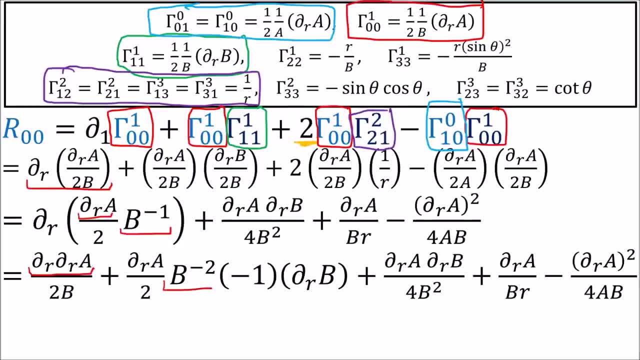 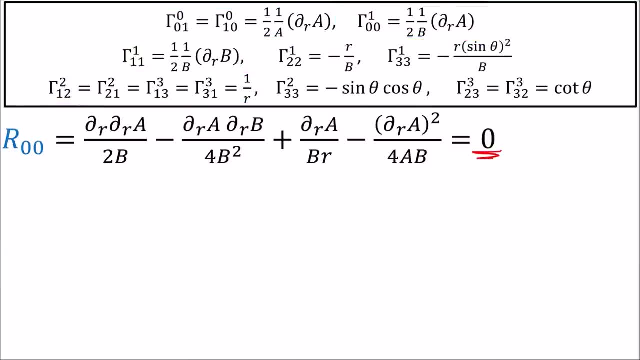 use power rule on b to the negative 1 to get b to the negative 2 times negative, 1 times a chain rule. derivative term Rewriting. we get this Now. remember all of this is equal to 0, since the Ricci tensor is 0 in our solution. To make this easier to read, I'm going to replace: 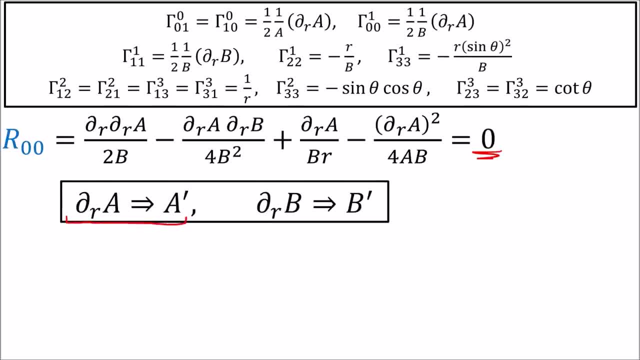 the partial derivative of a with respect to r with a prime and replace the partial derivative of b with respect to r with b prime. I'm also going to multiply the equation by a common denominator of 4ab squared r to get rid of the denominators. So that was r00.. For r11 and r22: 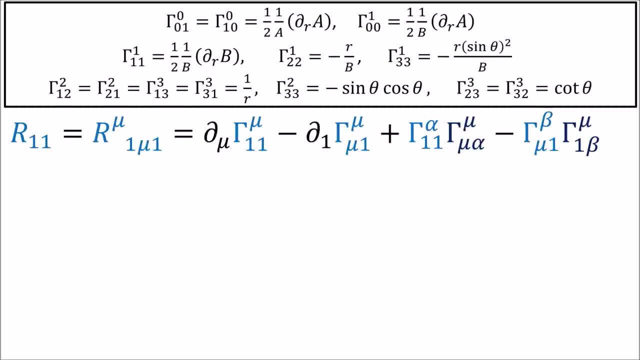 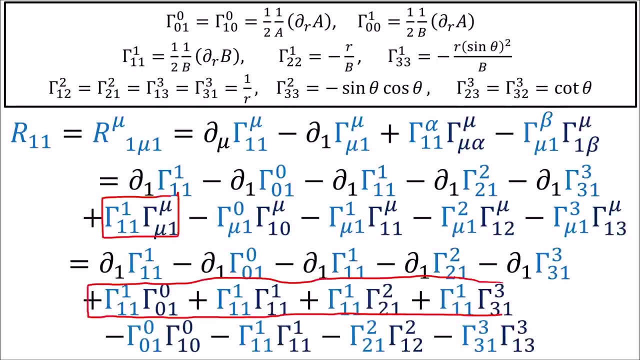 I'm just going to run through them quickly. You can pause the video. if you want to check the algebra For r11, we have mu equals 1 here and expansion to four terms: alpha equals 1, and alpha equals 2.. We get another expansion to four terms and mu equals 0,, 1,, 2,, 3. for the rest, 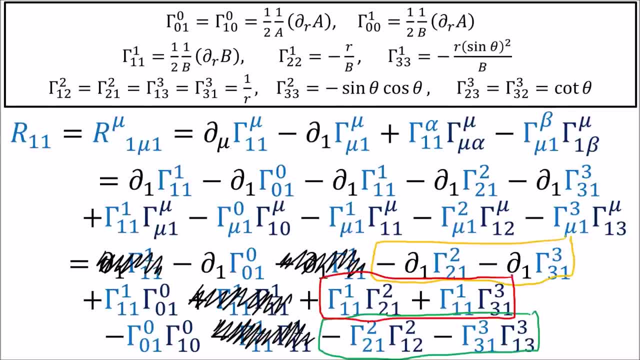 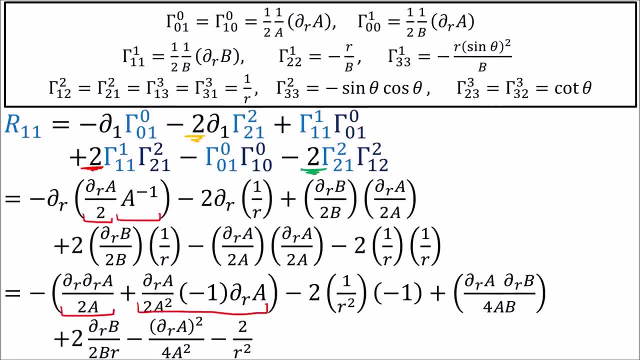 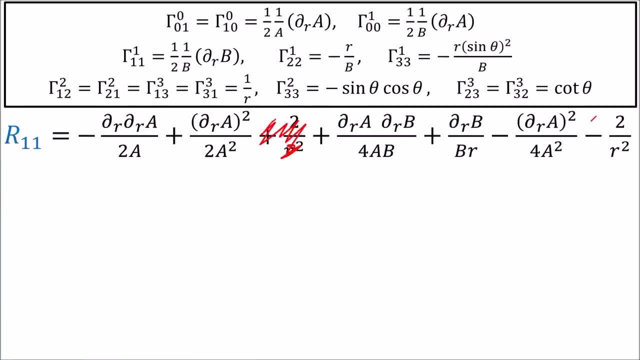 Then we do some cancelling and grouping of like terms. After subbing in the coefficient formulas. we need to do product rule on the first term and use power rule on 1 over r to get 1 over r squared times negative 1.. We can then do some cancelling and combine terms and we 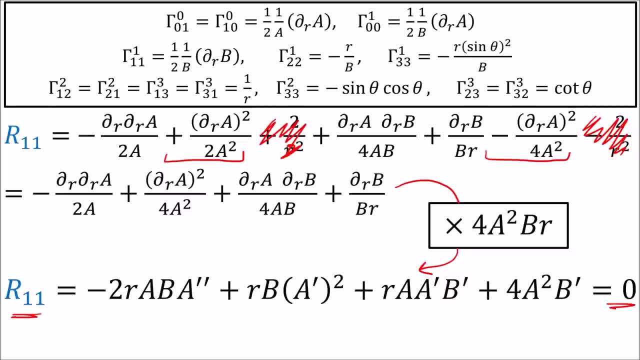 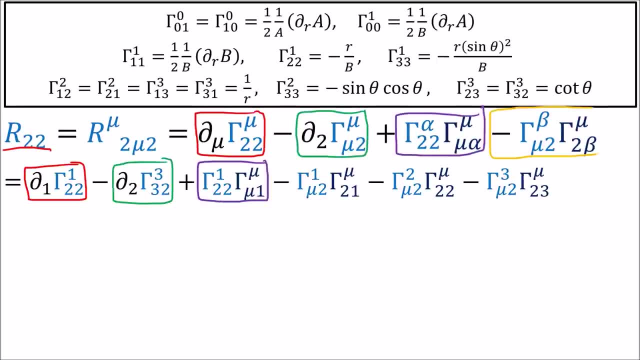 multiply by 4a squared br to get rid of the denominators For r22, we have mu equals 1, mu equals 3, alpha equals 1, and beta equals 1,, 2, 3.. This sum expands to four terms. 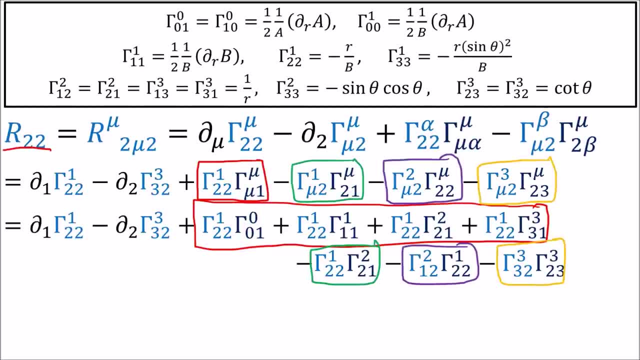 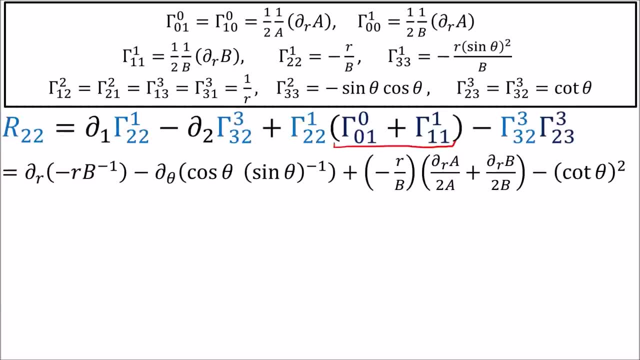 and then we have mu equals 2,, mu equals 1, and mu equals 3.. Then we cancel and factor like terms. After we sub in the formulas we have to do the product rule on r times b to the negative 1, and also cotangent, which is just cosine times sine, to the negative 1.. 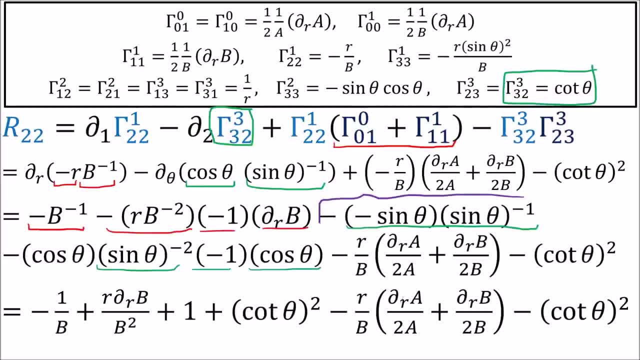 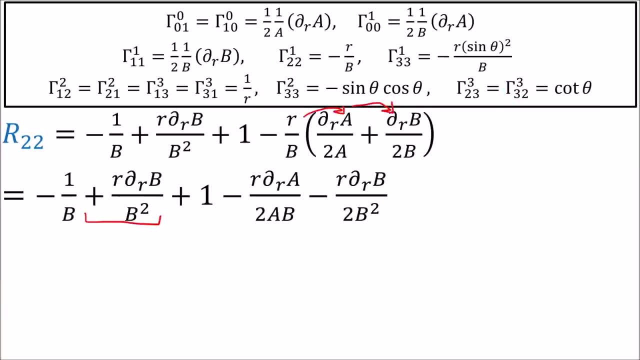 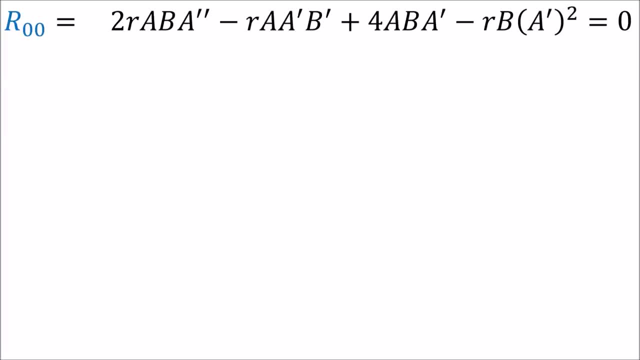 So we have product rule and product rule. This is just plus 1, and this is cotangent squared. So we cancel, distribute, combine and multiply by 2 times ab squared to get rid of the denominators. So all these Ricci components equal 0.. This means that if we add r00 and r1,. 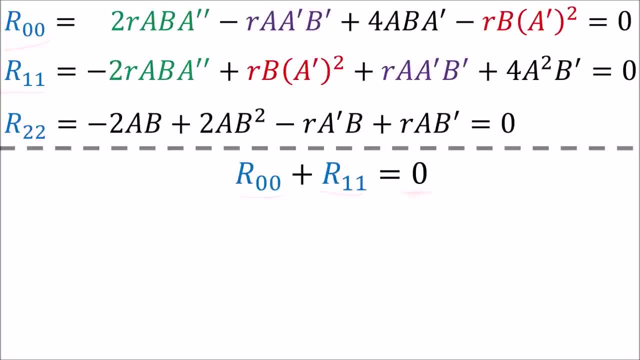 the result should be 0.. If we sum these terms in r00 and r11, these cancel, these cancel and these cancel, So we get 4a ba prime plus 4a. squared b prime equals 0.. If we cancel 4a from both terms, we get ba prime plus a b prime. This is just the product rule result. 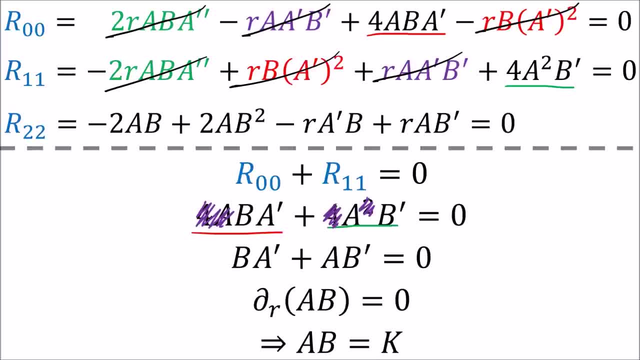 from the derivative of a times b, and since this derivative is zero, this tells us that a times b is a constant, which I'll call capital K. Now we know that, as the Schwarzschild metric goes out to, r equals infinity, it will. 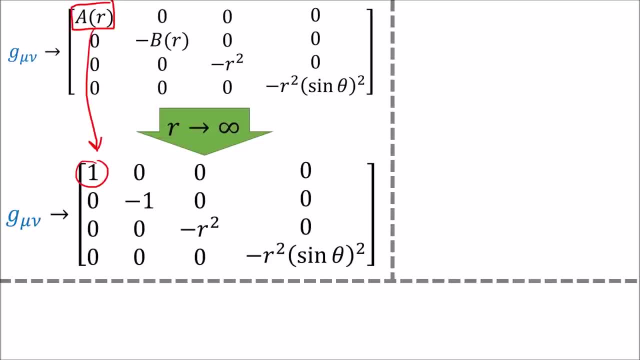 approach the Flat-Minkowski metric, where a equals 1 and b equals 1.. So in this limit, a times b equals K becomes 1 times 1 equals K And since K is the same constant for all r values, K equals 1. 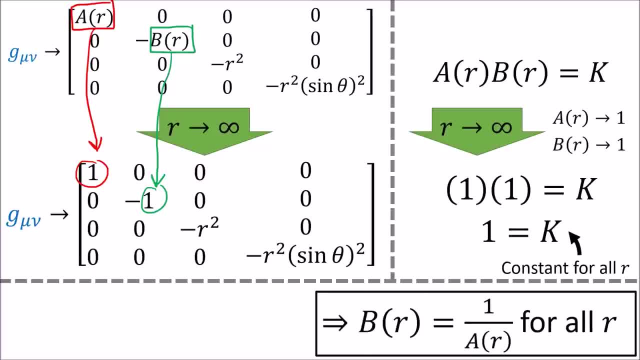 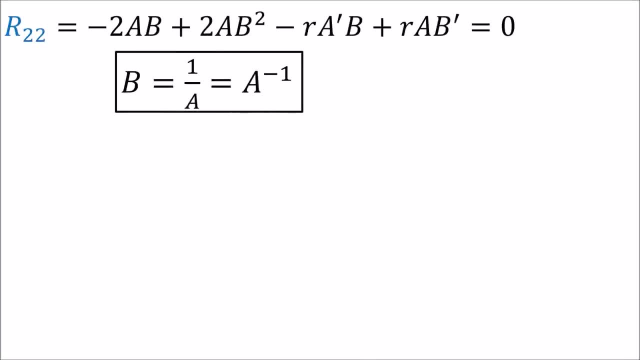 for all r. This means that b equals 1 over a for all r. So, knowing the R2-2 formula and that b equals 1 over a and that b prime is the derivative of 1 over a, which is negative a prime over a. 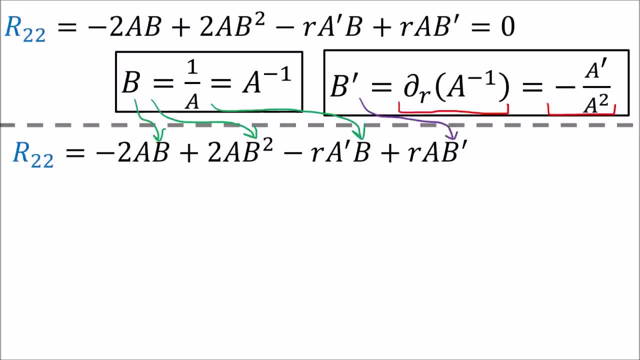 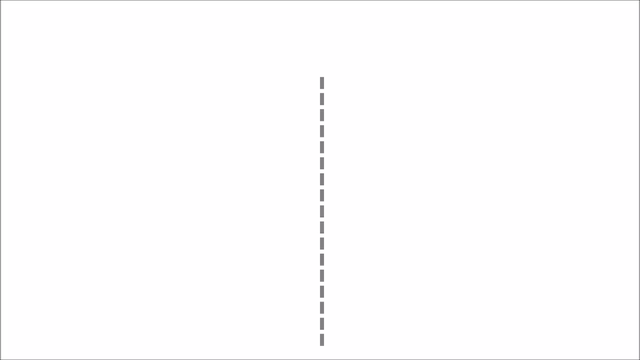 squared. we can substitute in for b and b prime. If we cancel factors of a and add these together, cancel the 2s and rearrange, we get the differential equation. r times a prime equals 1 minus a. The solution to this equation is a of r. 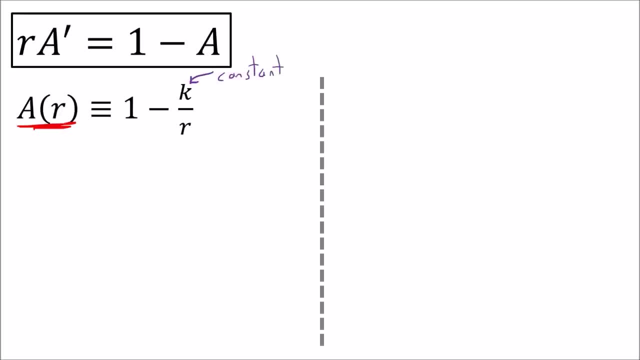 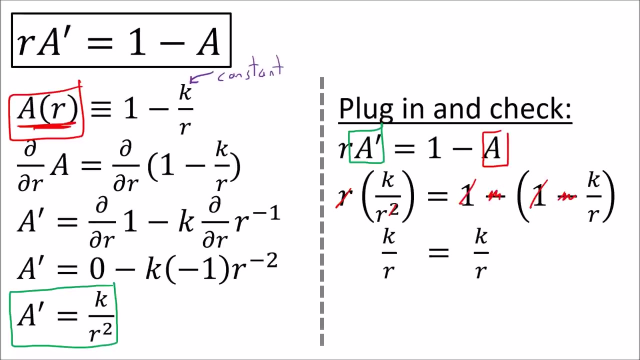 equals 1, minus a constant small k over r. If we calculate the derivative of a, we find that it's K over r squared. And if we plug a prime and a into our differential equation, r is cancelled here, 1's cancelled here and we get K over r equals K over r. So this solution. 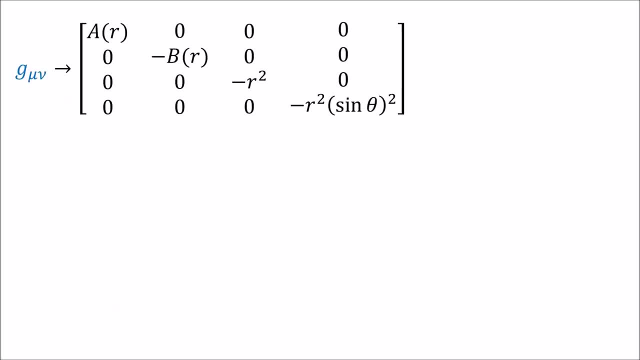 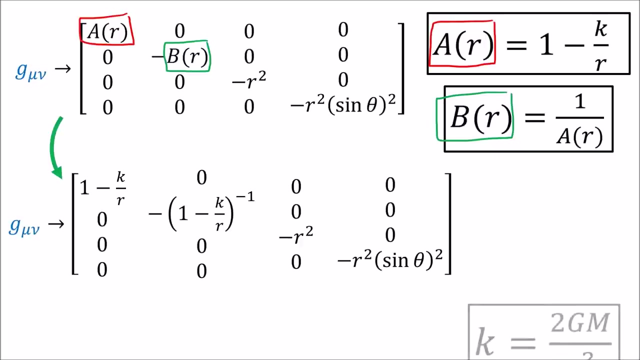 satisfies the differential equation. So we've solved for: a of r equals 1 minus k over r, and b is just 1 over a, So we have the form of the Schwarzschild metric. Now we just need to solve for the constant k, which ends up being 2 g m over the speed of light squared. 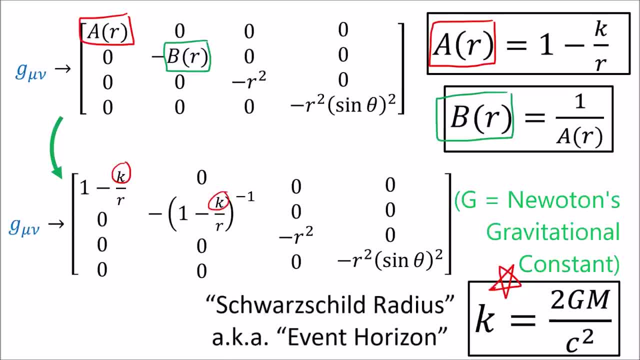 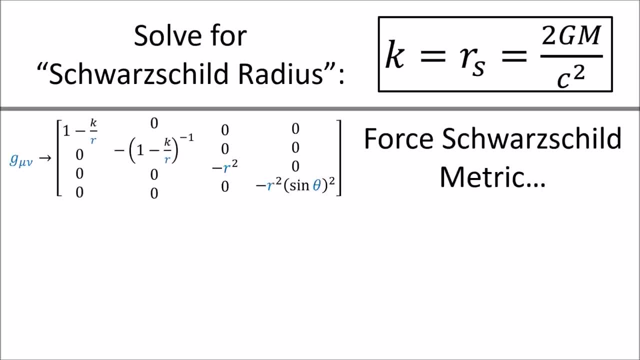 This is called the Schwarzschild radius or the event horizon of the black hole. We can solve for the lowercase k constant by forcing the Schwarzschild metric to reproduce Newtonian gravity in the limit of low velocity and weak gravity. For this part of the video, I'm going to use the Minkowski metric in Cartesian coordinates. 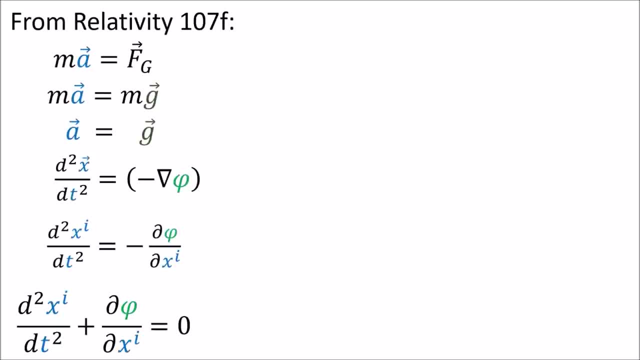 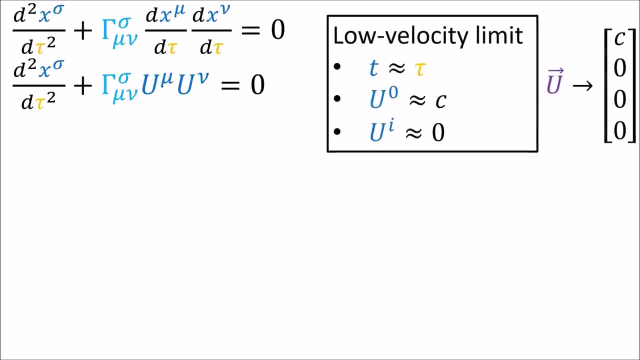 instead of spherical coordinates. I showed in Relativity 107f during the derivation of the Einstein field equations that we can force the geodesic equation to match the Newtonian equation for acceleration due to gravity In the limit of low velocity. the proper time is approximately: 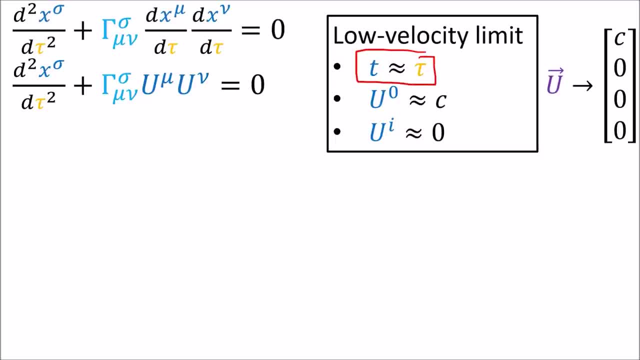 equal to the coordinate time t and an object's four-velocity vector components are dominated by the time component, which is basically c, with the other components going to zero. To get the geodesic equation to match Newtonian acceleration we need to use the Schwarzschild metric. 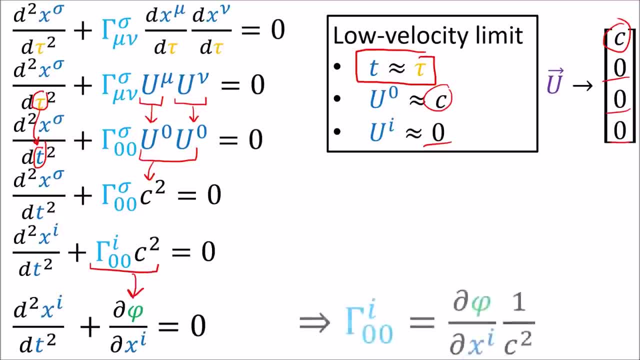 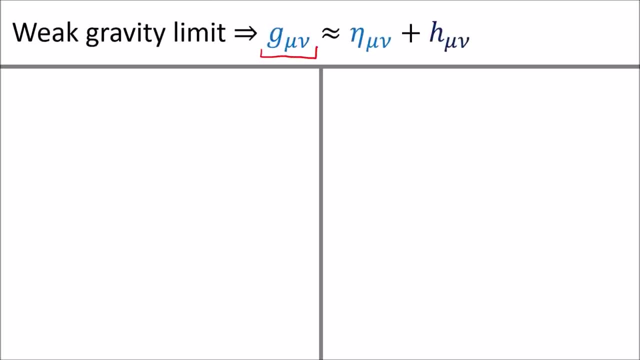 We need the i00 connection coefficient to be 1 over c, squared times the partial derivative of the gravitational potential phi in the i direction. Now, when we say we're taking the limit of weak gravity, this means that the metric can be written as a sum of the flat Minkowski metric, eta, plus a small change h, where the 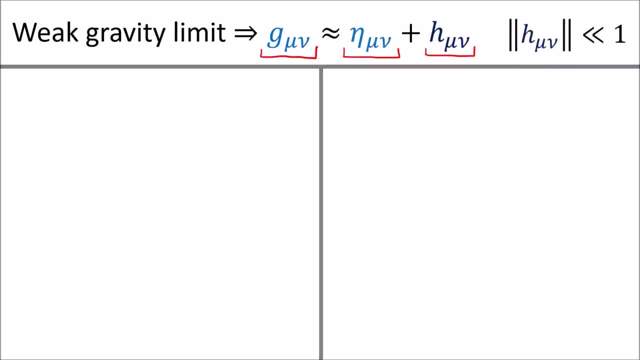 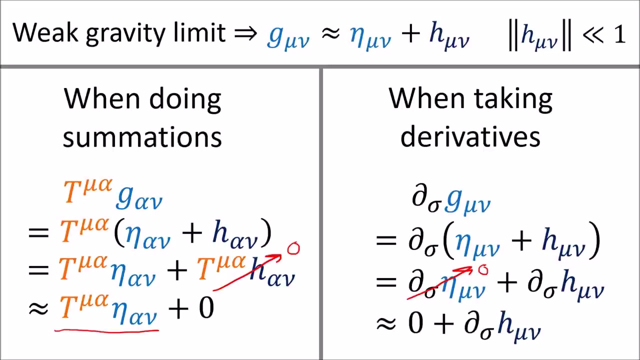 components of h are much less than 1.. This basically means that when we do a summation with the metric, the h part is small enough to be ignored. But when we take the derivative of the metric, we ignore the constant Minkowski part in Cartesian coordinates and only get 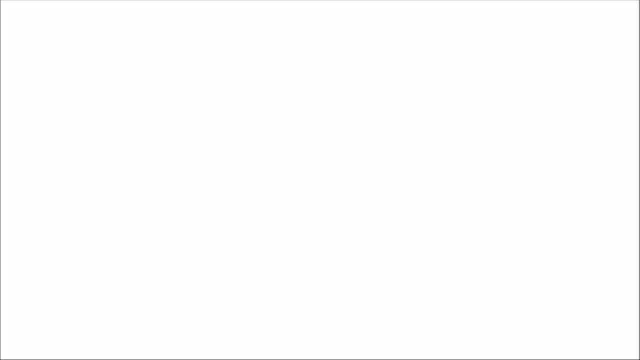 the derivative of the h part. So if we take the formula for the connection coefficients and look at the i00 case, this inverse metric can be approximated by the flat Minkowski metric and these metric derivatives are equal to the derivative of the h part. 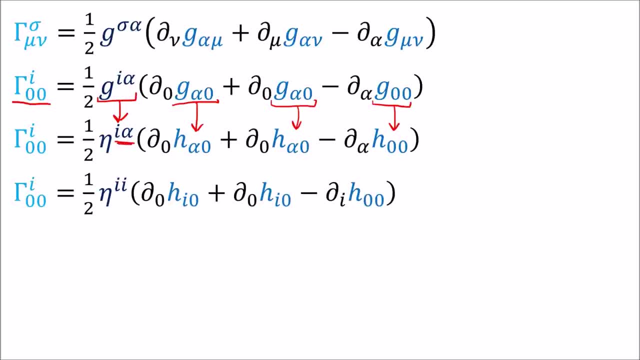 And since the metric is diagonal, we know this alpha index must match the spatial index i if we want the components to be non-zero. The first two terms are off-diagonal and go to zero, And the space-diagonal elements of the Minkowski metric are all negative. one in Cartesian. 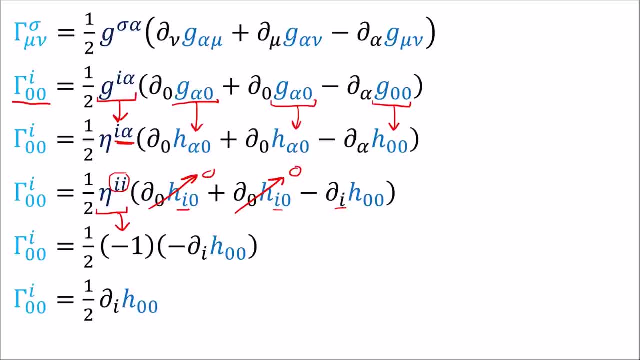 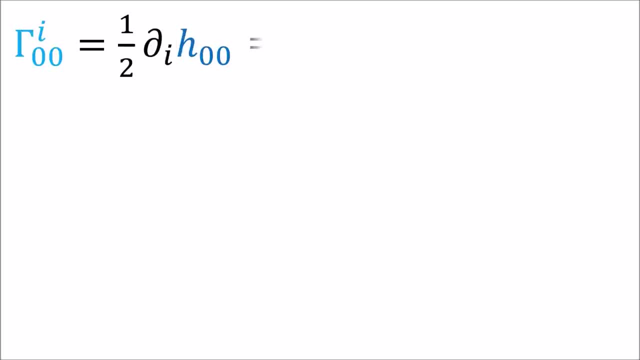 coordinates. So we're left with gamma i00 equals one half times partial i of h00. But recall that gamma i00 is just one over c squared partial i of the gravitational potential. If we remove the derivatives on both sides, we see that h00 is just two times the gravitational potential over c. 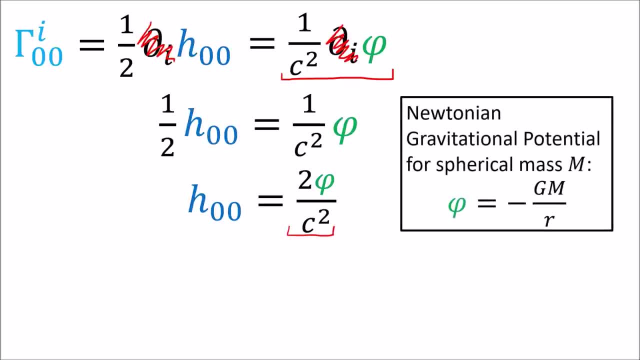 squared In Newtonian gravity, the gravitational potential for a spherical body of mass m is negative g times m over r. This is what gives us the standard Newton's law of gravity after taking the gradient and multiplying by a second mass. So h00 equals negative two gm over c squared r. 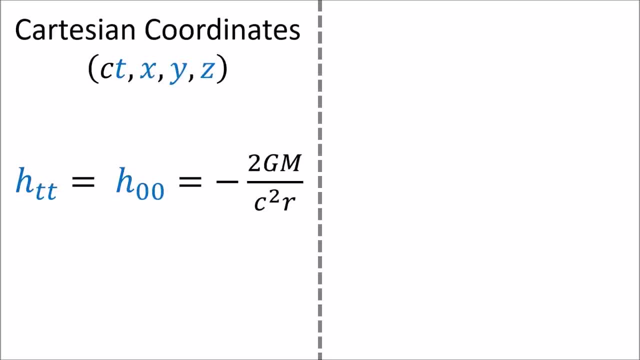 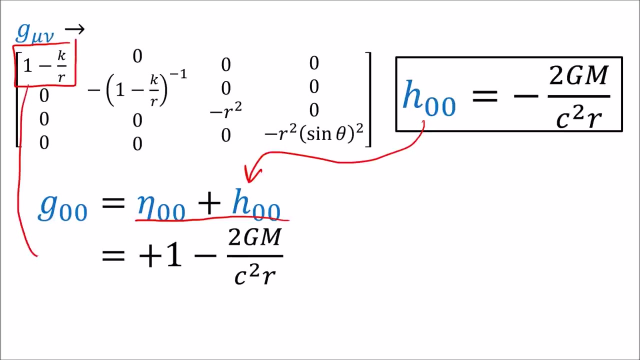 So, since we've solved for h00 in Cartesian coordinates, we've also solved for h00 in spherical coordinates, since both coordinate systems use the same time coordinate. Comparing this to the form of the g00 component of the metric that we've derived the constant small k. 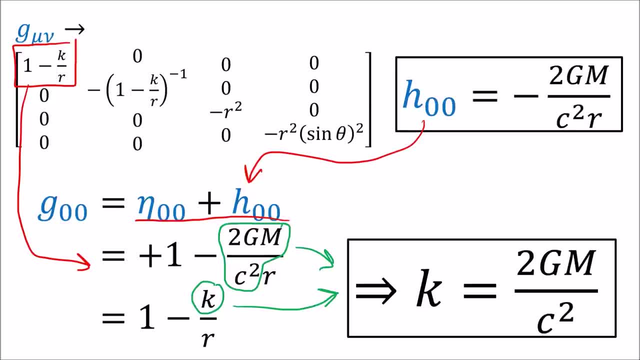 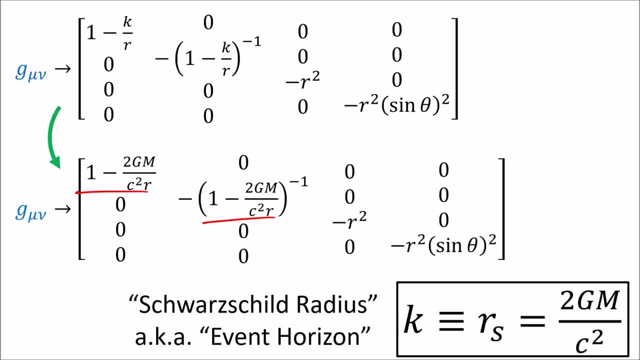 must then be equal to two gm over c squared, which we can plug into the formula for the g00 component as well. This component, two gm over the speed of light squared, is also called the Schwarzschild radius and is often denoted by r subscript s. This completes the derivation of the Schwarzschild. 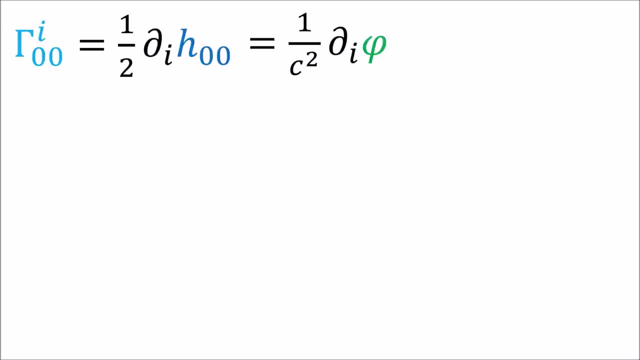 metric. One last thing before I conclude. A few slides ago, some people might point out that cancelling derivatives on both sides of the equation would be better than canceling them. So, for example, if I wanted to cancel the derivative on both sides of the equation, I'd have to use the 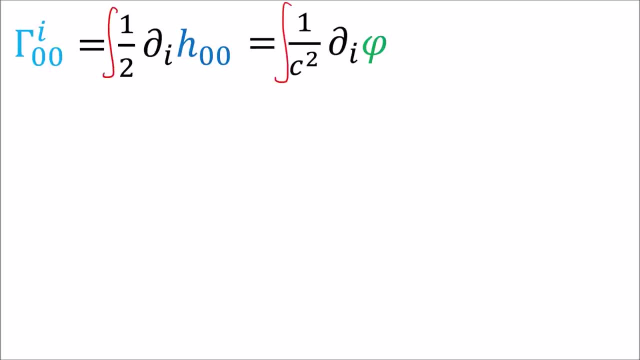 Schwarzschild radius, which is the same as the derivative on both sides of the equation, And the correct thing to do is to integrate both sides, which gives an additional constant of integration, giving this for h00 and this for g00.. But since we want the metric to reduce to, 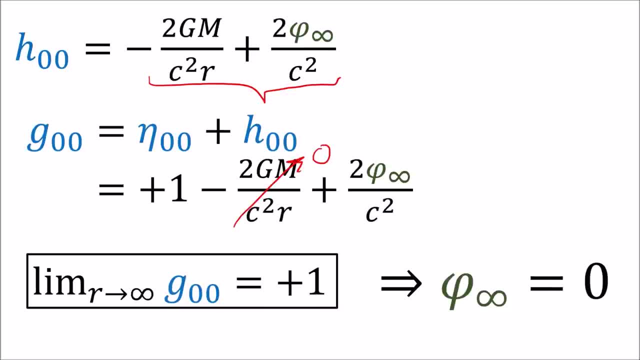 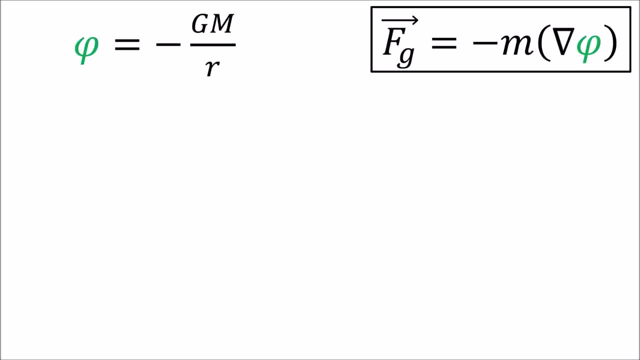 the flat Minkowski metric. as r goes to infinity, we're forced to set this integration constant to zero. This is similar to how the Newtonian gravitational potential negative gm over r can also have an extra constant added on to it, because the constant goes away when we take the. 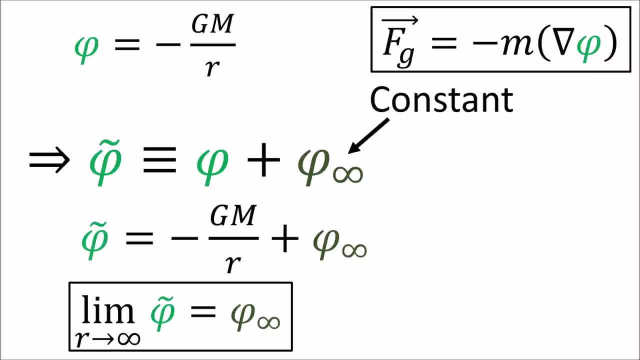 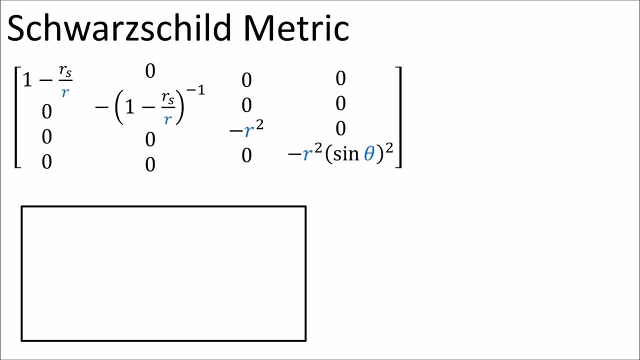 gradient. This constant is the potential's value at infinity. So this value must be zero if we want the potential to be zero, infinitely far from the mass. So, to summarize this video, we derived the Schwarzschild metric, which is the spacetime metric for a spherically symmetric uncharged 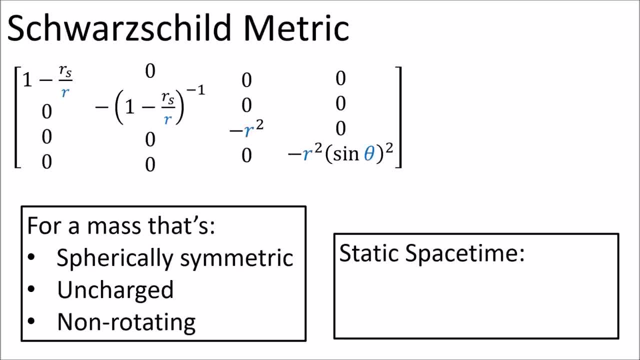 non-rotating mass, together with the addition of the Schwarzschild metric, which is the space-time additional assumption that spacetime is static, meaning in our coordinate system the metric doesn't depend on time and also spacetime doesn't change when we